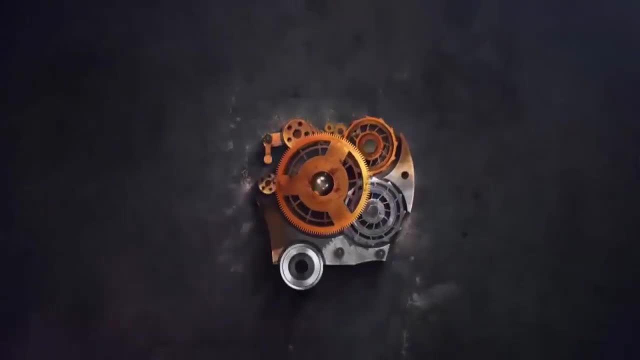 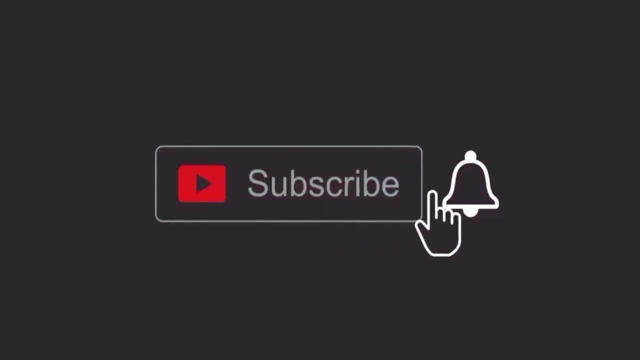 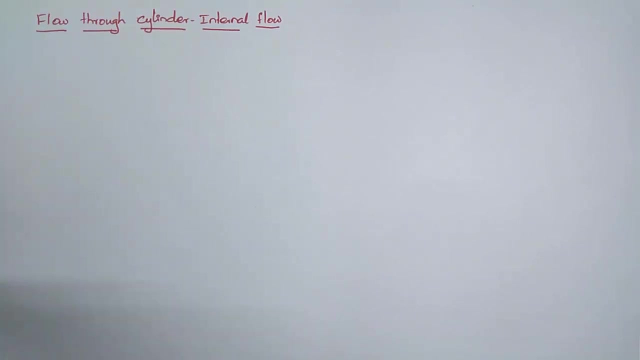 Hello everyone, welcome you all back. In this video we are going to see internal flow by forced convection, that is, flow through a cylinder by forced convection. Now let me explain. before going to the problem, Let me explain the boundary layer development inside a pipe or inside a 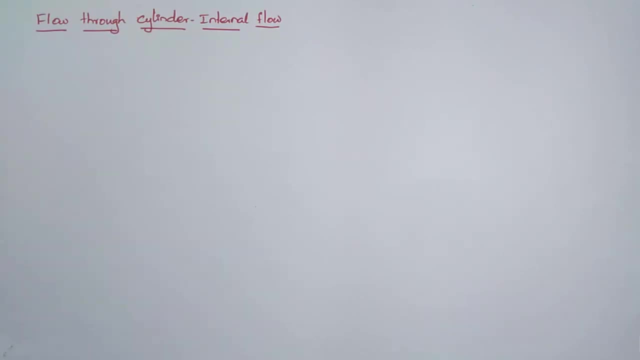 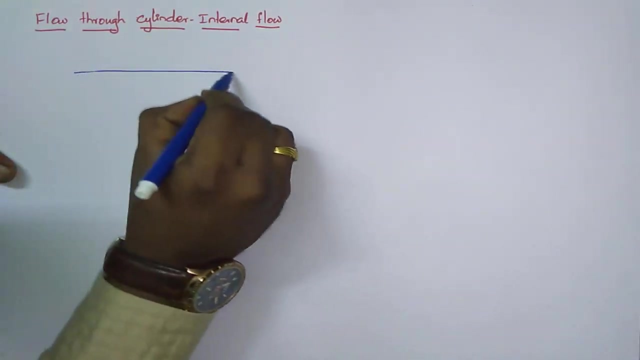 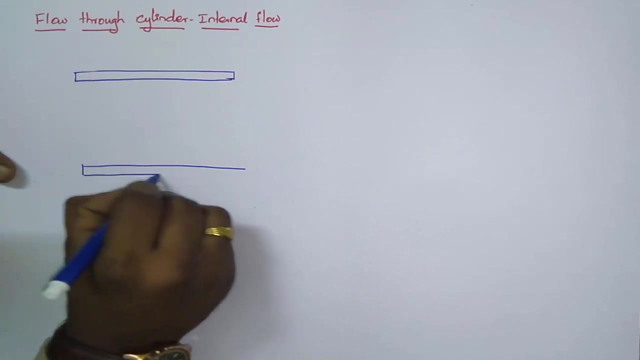 cylinder. that is internal flow, right. So now consider a pipe like this. If you, if you have the cross section of the pipe, you will get a cross section of the pipe like this: This is your top wall of the cylinder and this is your bottom wall of the cylinder. Now consider the flow of. 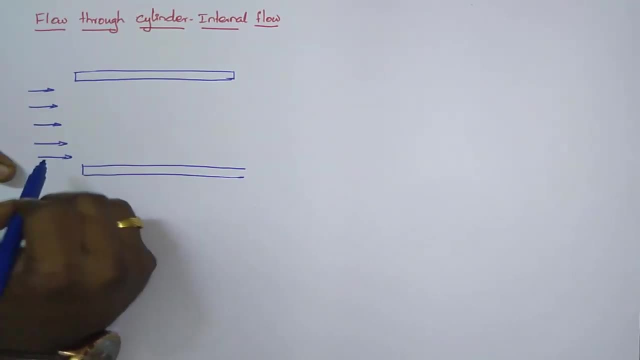 the fluid, that is, the fluid is flow in this direction with a velocity of u infinity. that is, the fluid velocity is u infinity. Once the fluid reaches the entry point of the cylinder, because of the friction motion between this plate surface and the fluid movement, the boundary layer starts. 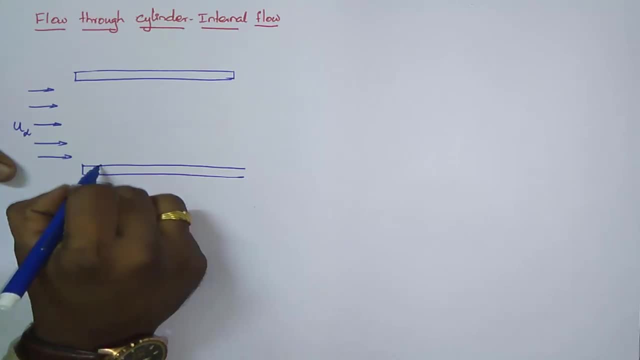 to change and the surface of the wall, the velocity is equal to zero. So here u equal to zero. Then the velocity starts to increase like this, and it will attain the? u infinity value. Here the velocity is u infinity. Similarly, throughout the wall, that is, if it is a cylinder, throughout the wall. in the 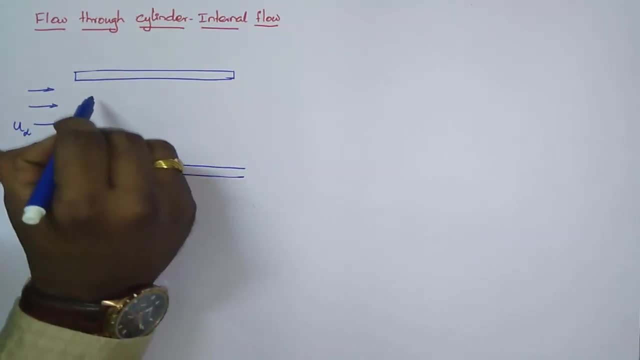 sense. if you cut the cross section, you will get the same thing in opposite direction also. Okay, like this, you will get the same thing in the opposite direction also. So now here, the velocity will be u infinity. Similarly, at some distance from here, you can see, you can observe a velocity. 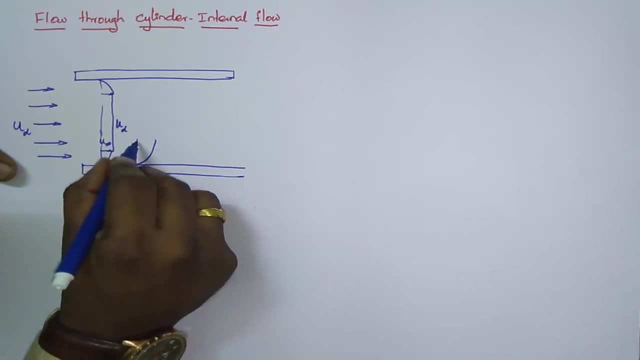 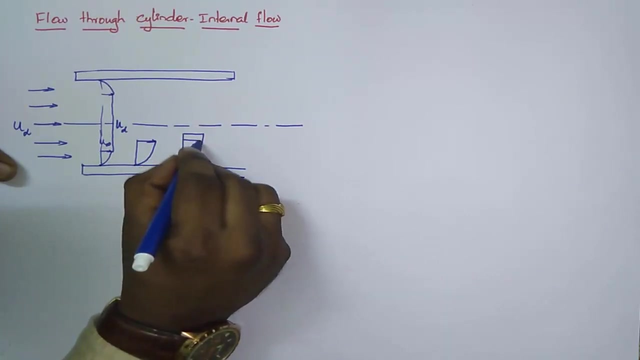 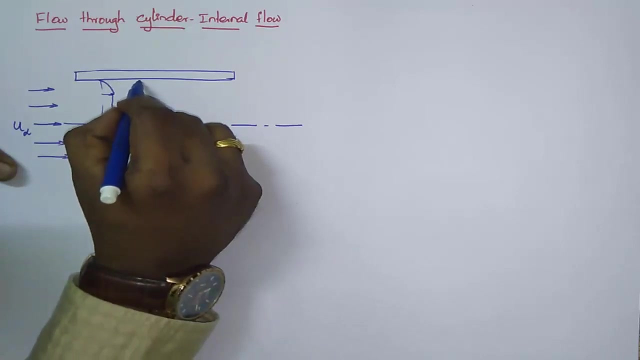 profile like this: This is your center line of the cylinder. In some more distance you will get a velocity profile like this. So this is your velocity profile, right. Similarly, in the in this, here in this wall also, you will get a cylindrical profile that is velocity profile like this. So here it will. 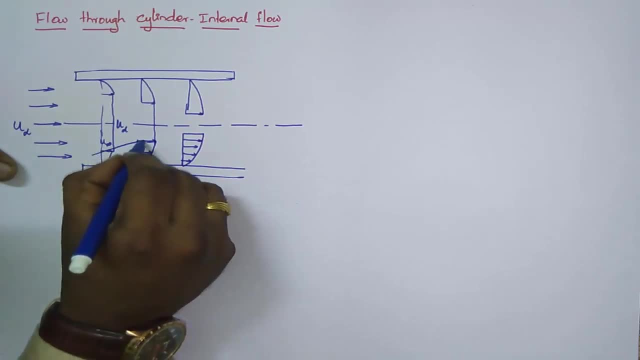 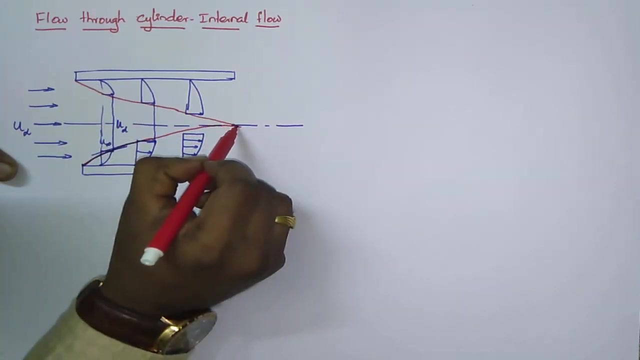 be a flat curve. So if you connect all these points, you will get the boundary layer development. you will get the boundary layer development just like this, In all the direction. you will get the boundary layer direction like this: At this point, these two boundary layer thicknesses matches to 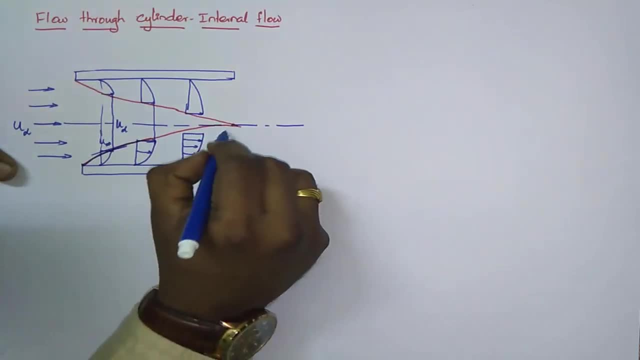 each other, and there the velocity profile will be like these. Similarly in the opposite direction also, the velocity profile will be like this: Now, after starting the cylinder, signed it. now you will visit the cylinder like this- and this will be your very first cylinder- roughly like this. Similarly in the opposite direction also, the velocity profile will be like this, Now after starting the cylinder. like this, However, the circularбо. 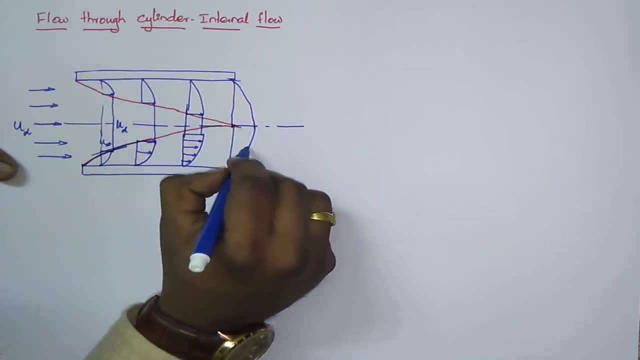 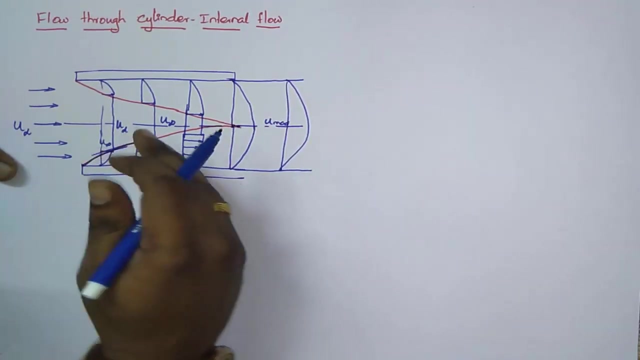 Now, if you consider this as the, here the velocity will be U infinity and at this point the velocity will be U max. Now, if you consider anywhere in the length of the pipe, the velocity profile will be similar, That is, the velocity profile will be constant throughout the length of the plate, throughout the length of the cylinder. after this point, right, 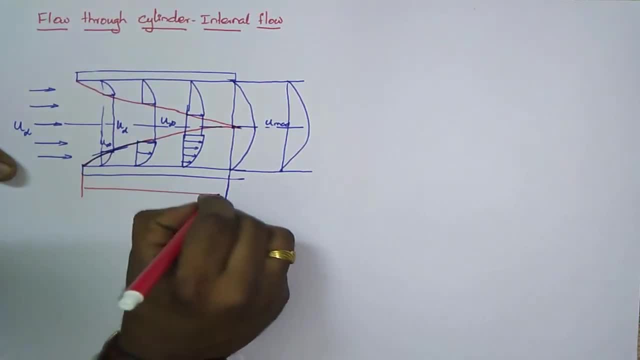 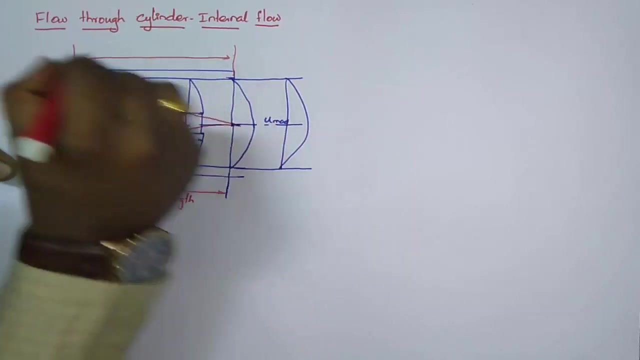 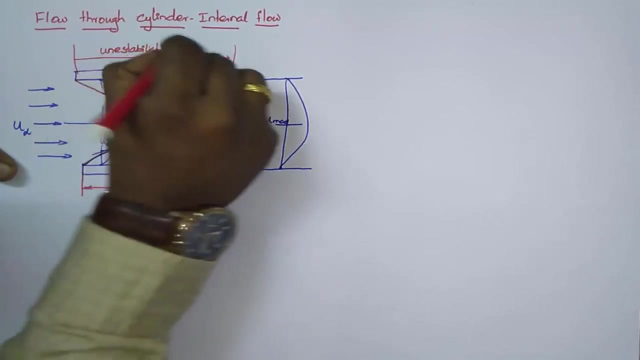 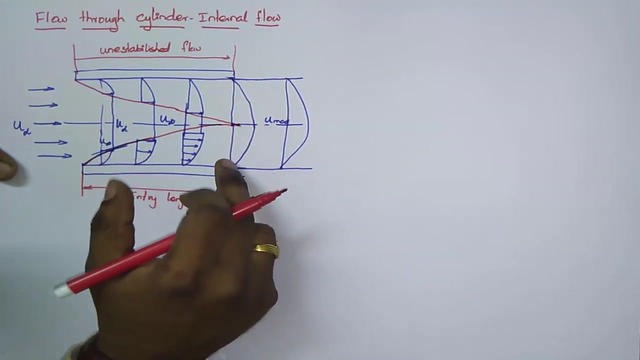 So up to this point it is called as entry length or entry region. okay, So up to this the flow is called as unestablished flow. So after this point the velocity profile develops fully. that is, the velocity profile develops completely. 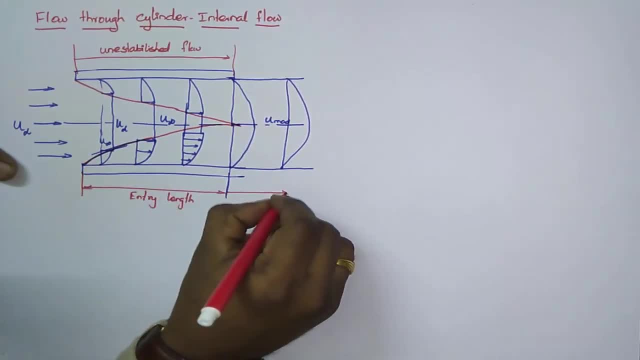 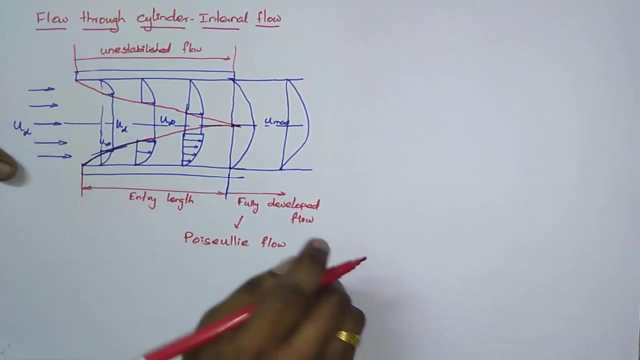 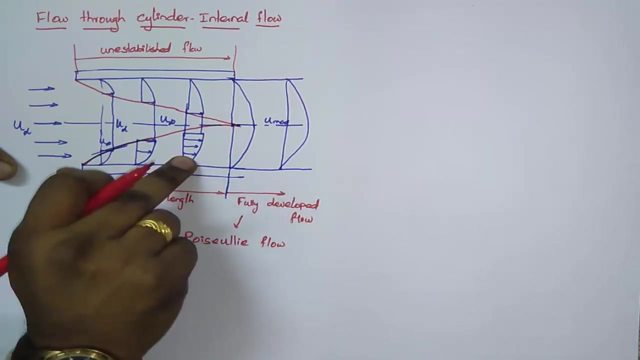 So after this point it is called as fully developed flow. fully developed flow or the fully developed flow can be called as poiseuille flow. Now you know what is entry length, what is fully developed flow, what is your velocity profile. and after fully developed flow it will be U max. and U max will not be equal to U infinity, that is input velocity. 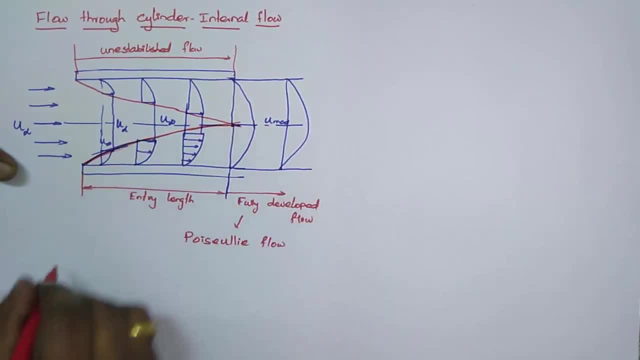 This is your boundary layer. So we have seen now for flat plate, The boundary layer thickness will be like this: After this it will be laminar, After that it will be turbulent. So the same phenomenon occur in the cylinder also. 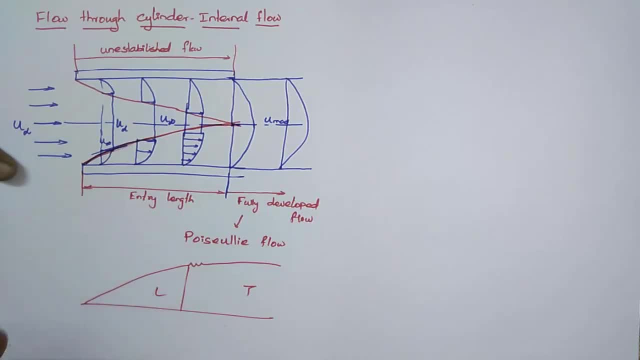 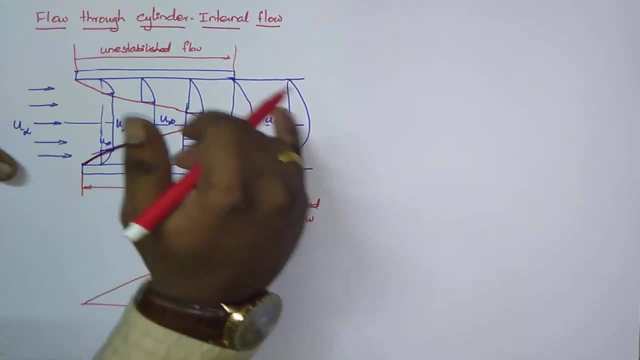 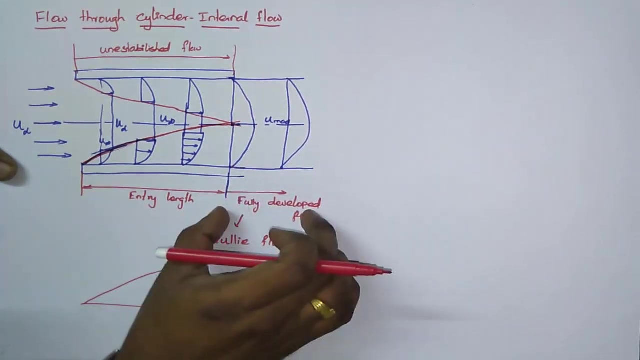 But in the cylinder in all the direction the velocity profile takes place and at some distance all the velocity profile converges at one point And after that point the velocity will not change at any point of the length. So that flow is called as fully developed flow or poiseuille flow. 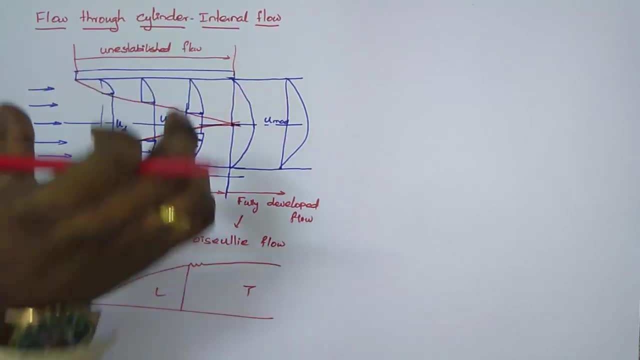 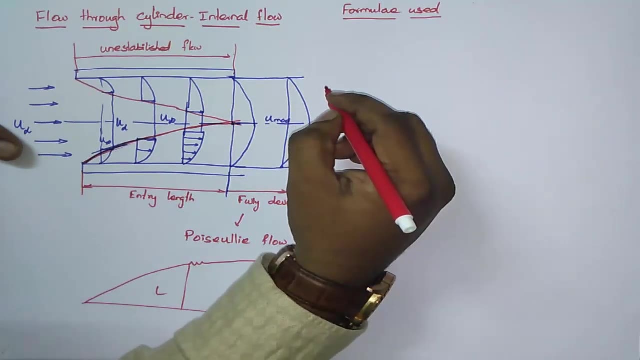 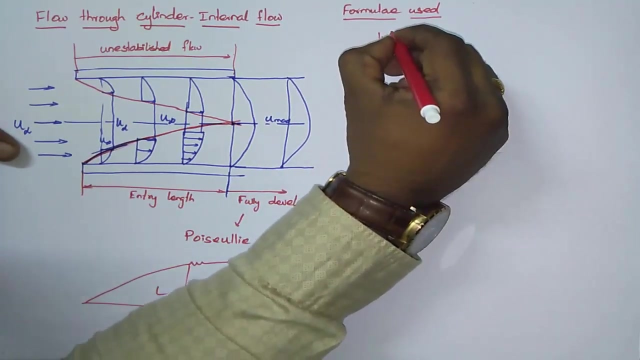 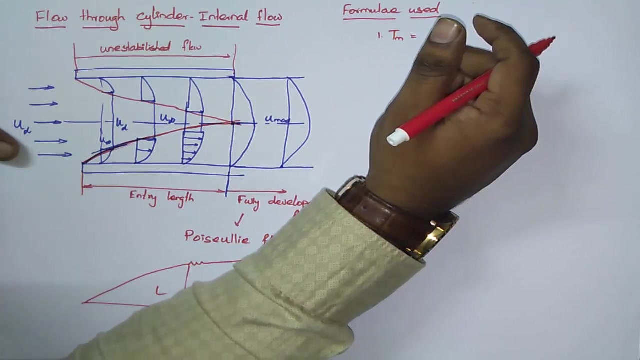 Before fully developed. It is called as established unestablished flow, or that length is called as entry length. Now I will give you the formulas which are going to be useful in solving the problems on internal flow Right. So first formula is T, mean temperature, where in the external flow over a plate we have find out the film temperature. 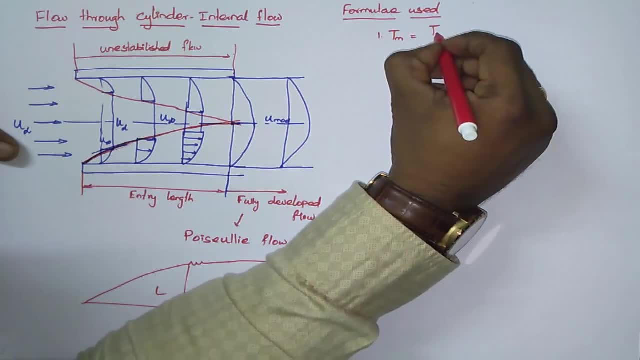 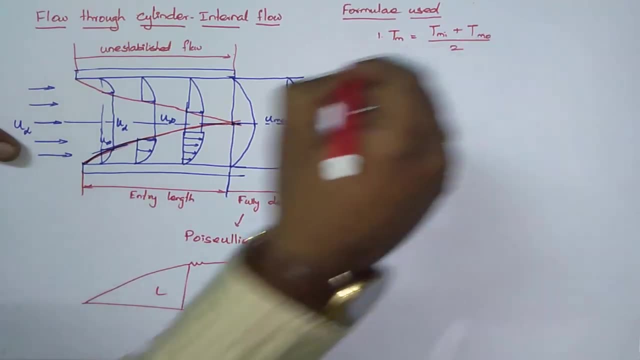 No, Here we are going to find out the T mean temperature, which is equal to T mean input temperature Plus T mean outlet temperature divided by 2.. These two temperatures will be given in the problem itself. usually The second thing is R E. 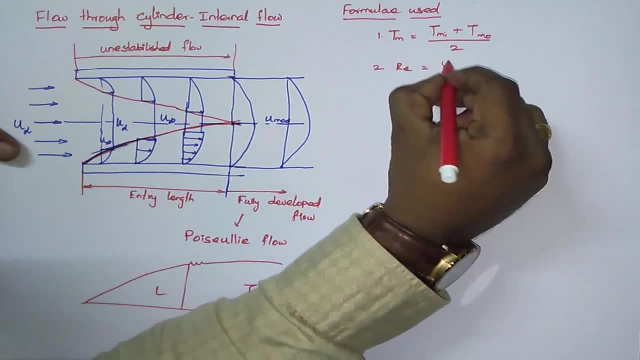 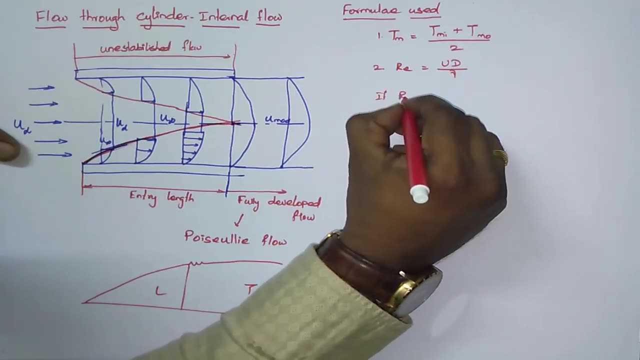 Reynolds number formula is here. it is internal flow. No, So U L. instead of U L we are going to use U D divided by nu. Okay, If R E is less than 2300, then the flow is laminar flow. 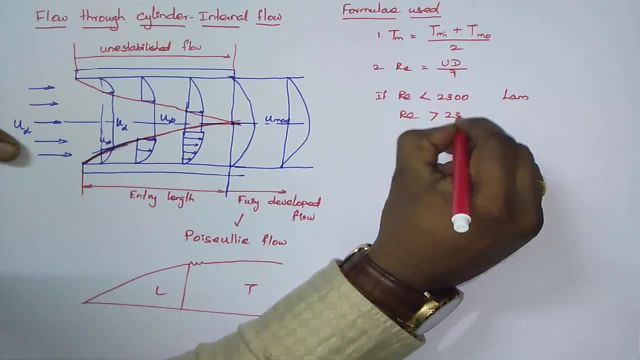 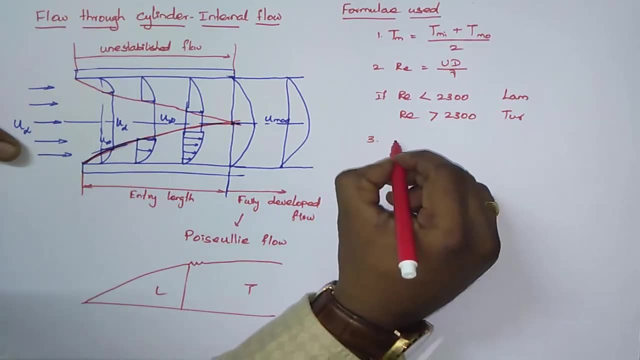 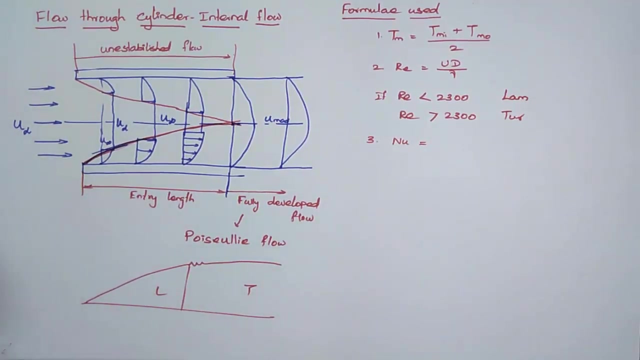 If R- E is greater than 2300. Then the flow is called as turbulent flow Right. The third formula is you have to take the Nusselt number formula from the data book. Right In the data book, from the index page you just find out the internal flow pages. 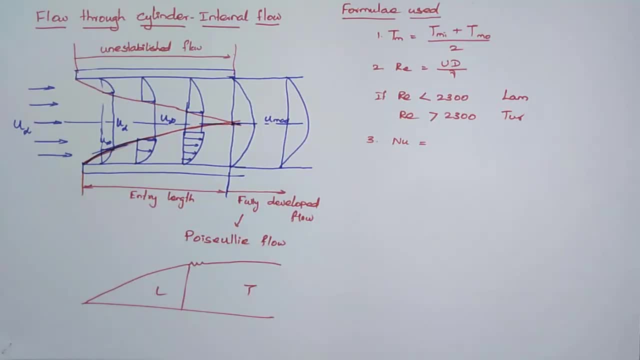 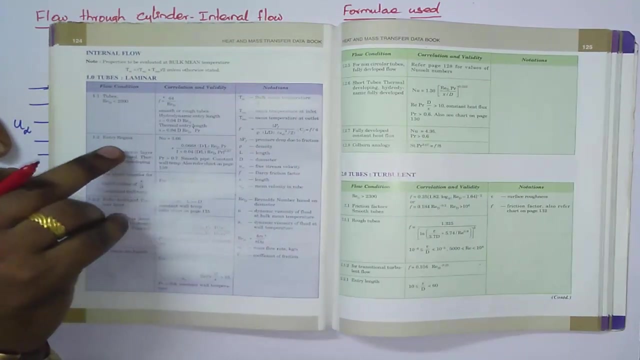 The internal flow pages are available in page number 124.. Right Page, number 124.. You can find out. So this is your page number 124.. Okay, In page number 124, you can find out the Nusselt number equation in the entry region. 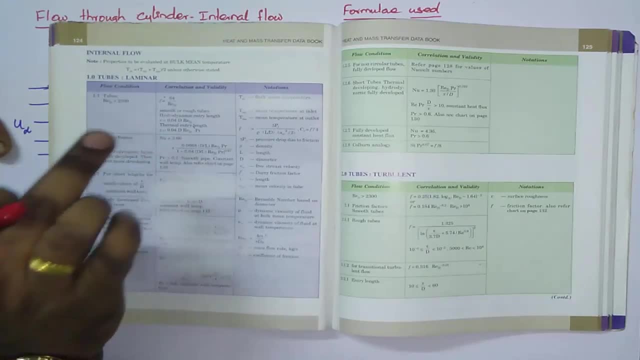 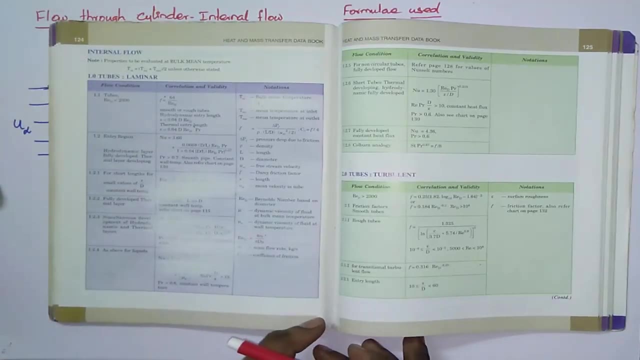 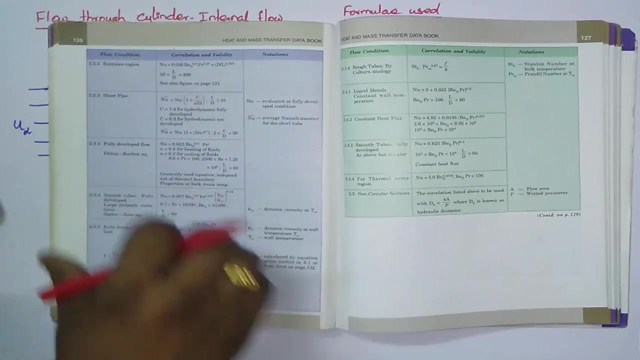 Nusselt number equal to 3.66.. This is the only formula you have to take for a laminar condition. So nu equal to 3.66.. Similarly for turbulent flow. here the turbulent flow formulas are given. Here you can. for laminar flow, this is the only equation you have to take. 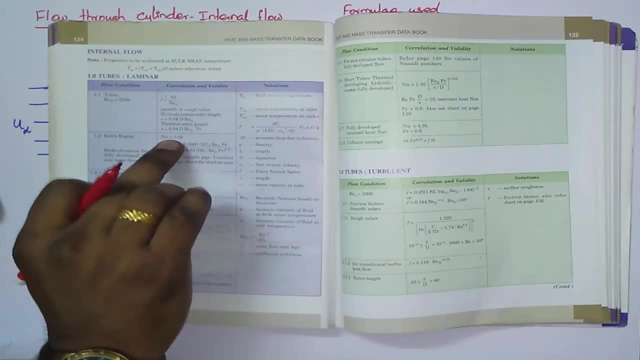 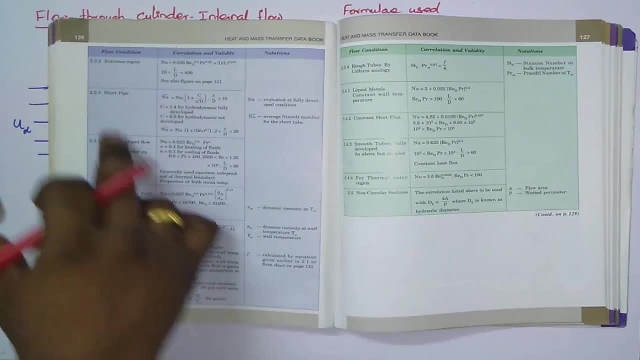 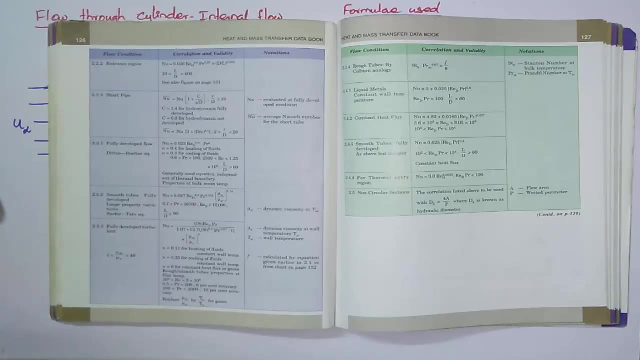 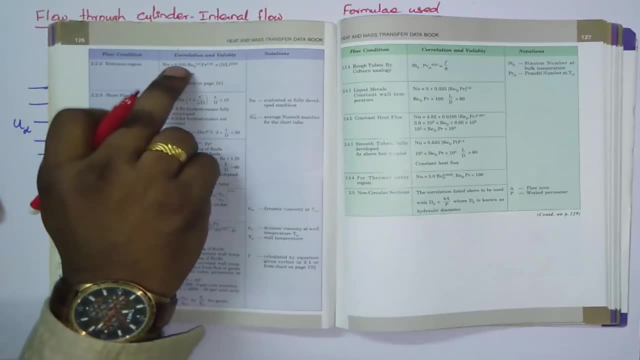 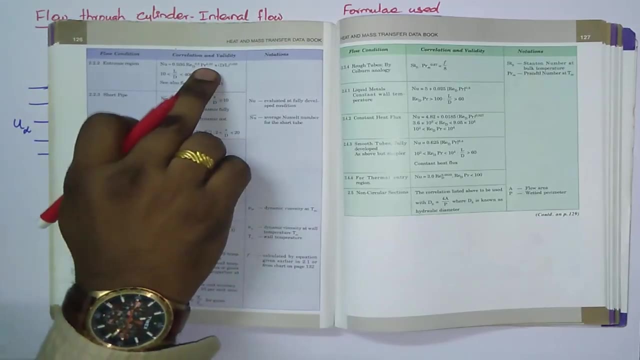 That is for the entry length. the formula will be nu equal to 0.036, RE power: 0.8. PR power: 0.33.. Okay, This is the entry region formula and the condition for the entry region is the L by D ratio should. 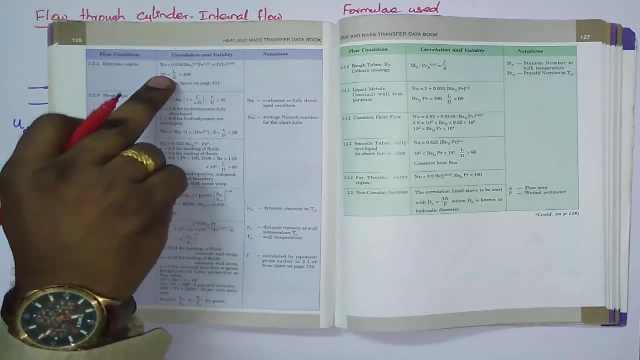 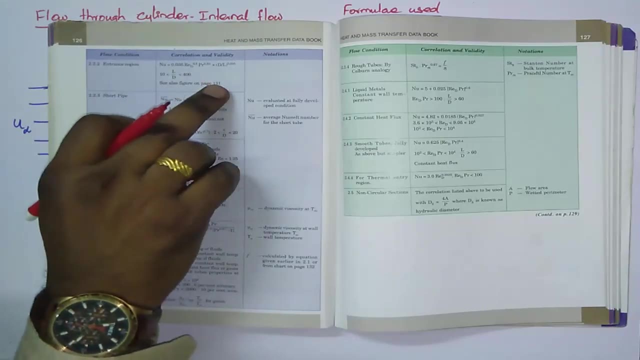 be less than 0.036.. than 400 and greater than 10, right? so if you find out the L by D ratio when the L by D ratio is between 10 to 400, then you can assume that the formula, the point, is in the entrance. 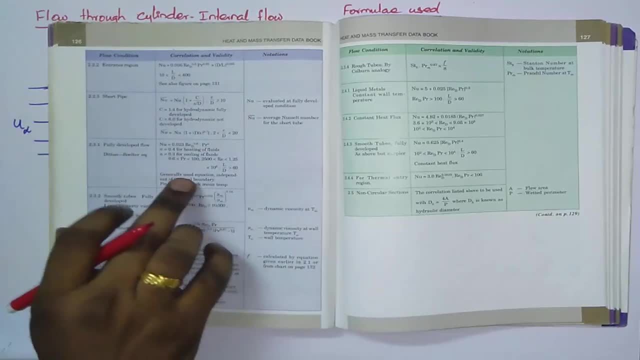 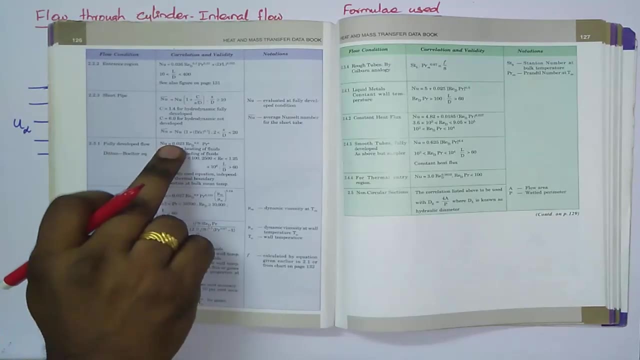 region and you can use this formula right similarly for a fully turbulent flow. so fully developed turbulent flow. the formula is given here: nu equal to 0.023. Re power, 0.8 Pr power. n. n equal to 0.4 for heating, n equal to 0.3 for cooling. right the conditions given here. 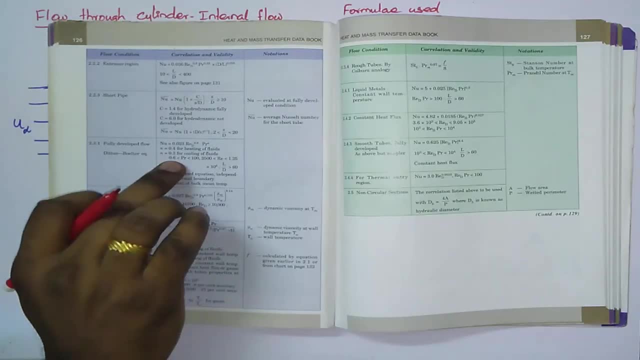 are Prandtl number should be less than 100 and greater than 0.6. similarly, the another condition is L by D ratio must be greater than 60, right? so first find out if it is a turbulent flow, find out the L by D ratio. if the L by D ratio is greater than 60, then you. 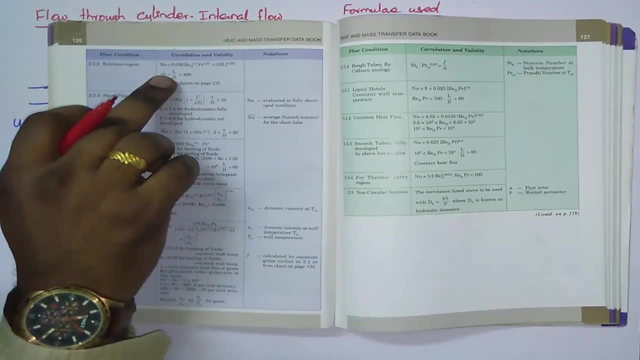 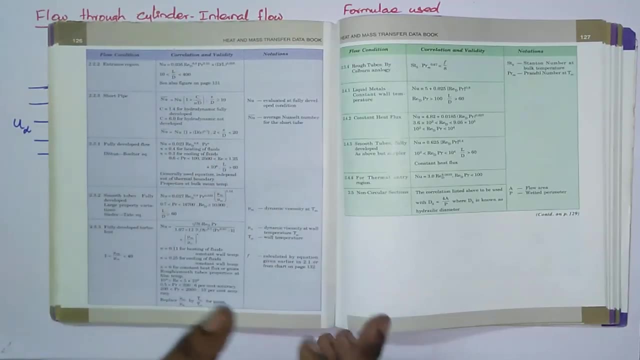 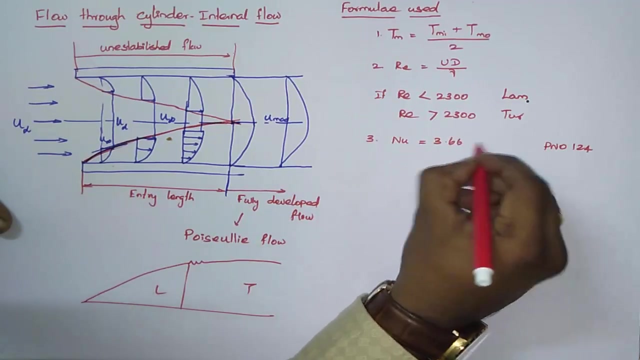 can come here. if the L by D ratio is 10, between 10 and 400, you can take this formula, and the Prandtl number also plays a vital role. we will see in detail while solving the problem right. so nu, equal to 3.66 for laminar flow in the fourth point, for turbulent flow. 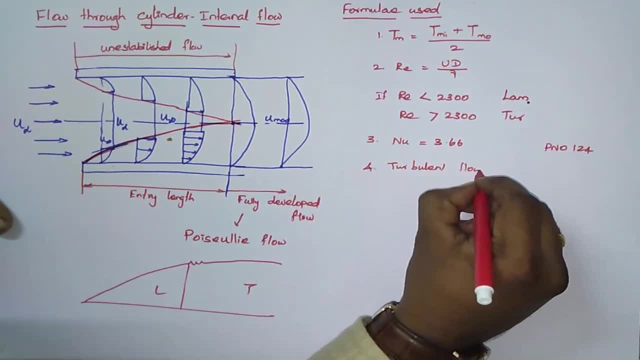 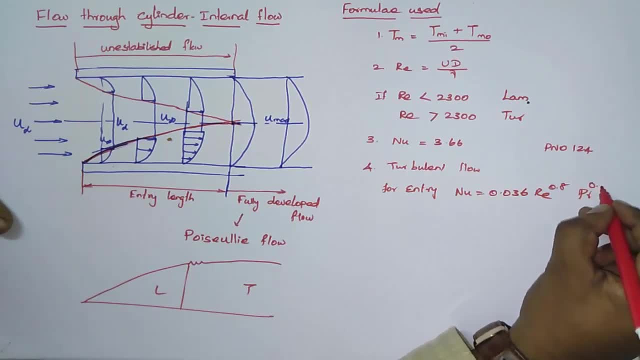 Re power: 0.036 Re power- 0.036 Re power- 0.037 Re power- 0.067 Re power- 0.037 Re power- 0.037 Re power: 0-12- 0.08 Re power- 0.33- 0.033 Re power- 0.033 × d. debate by L: the whole power. 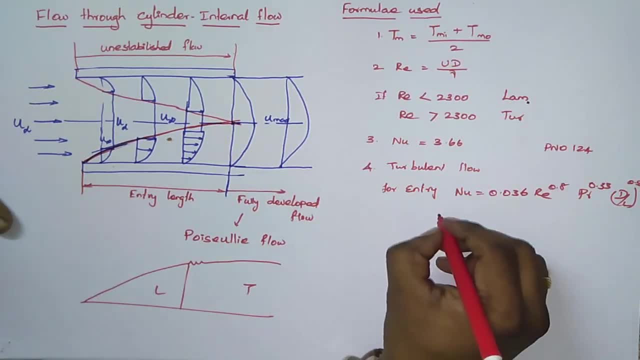 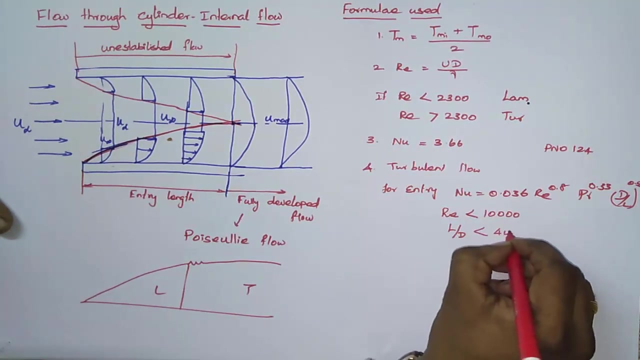 0.55. okay, this formula is valid when R唉nis number is less than ten thousand and L by D ratio must be less than four hundred and greater than 10, correct? So now the problem: what are you think, right? this is also a huge problem. 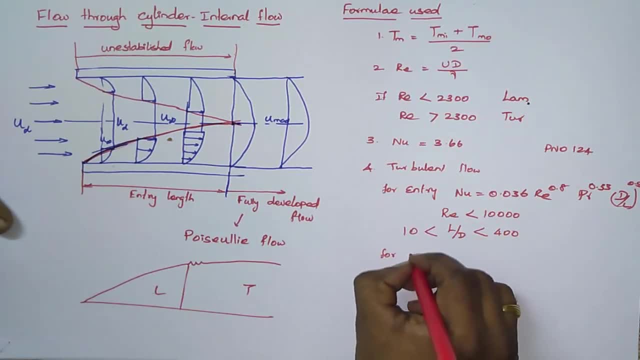 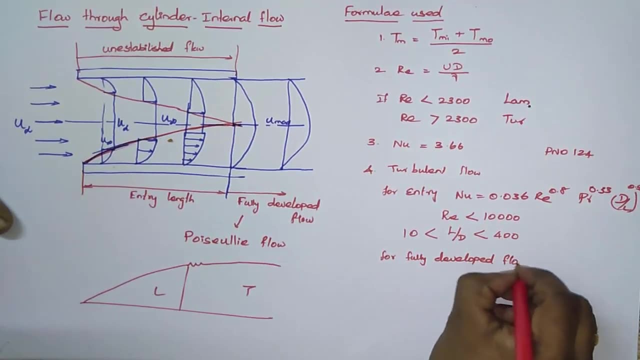 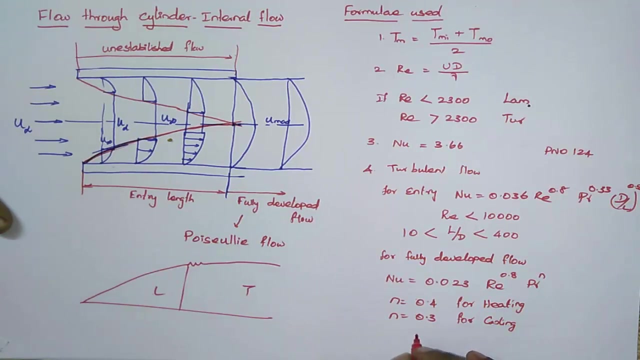 Then for fully developed flow. for fully developed flow, Nusselt number is equal to 0.023, Re power 0.8. Pr power N. N equal to 0.4 for heating, N equal to 0.3 for cooling, And the conditions for these will be: the L by D ratio must be greater than 60.. 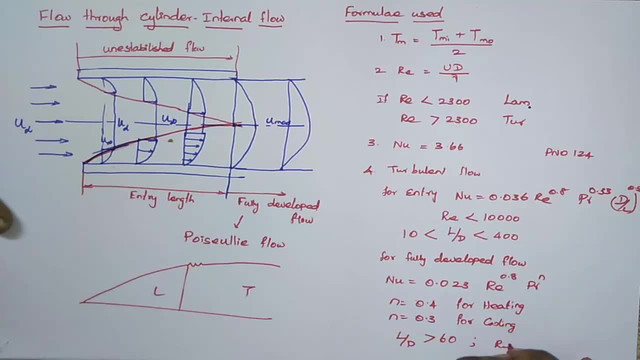 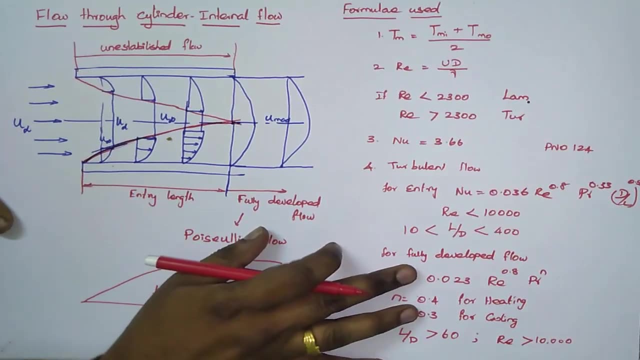 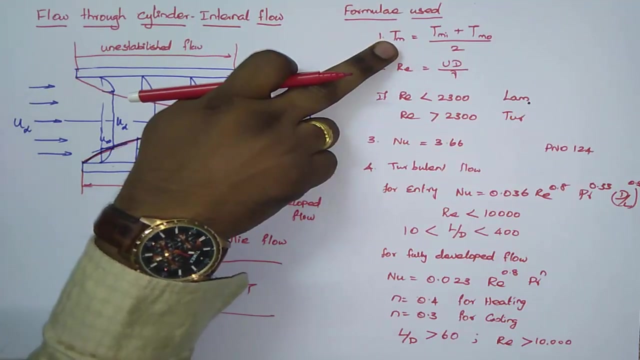 The second condition is Reynolds number must be greater than 10,000.. So once when you start to approach the problem, first to find out the T mean temperature and at the Tm take the properties of the dry air or water. Then, next step, you have to find out the Reynolds number value. 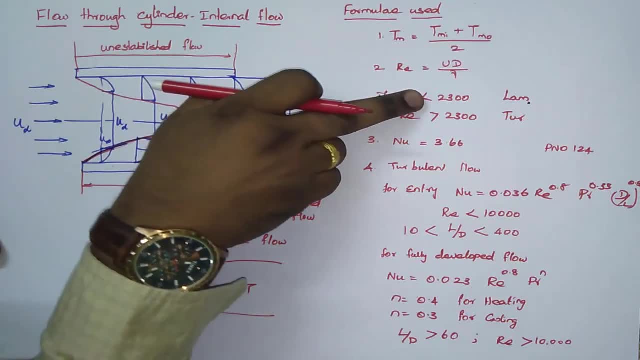 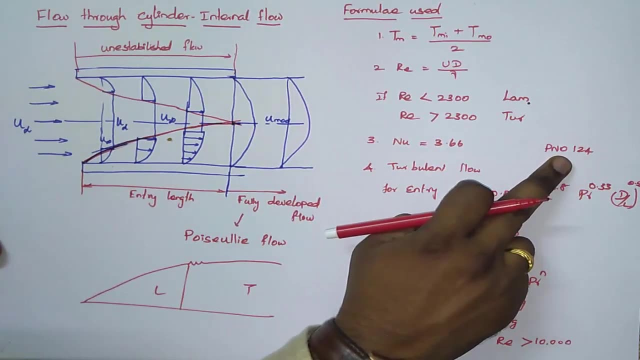 If the Reynolds number value is less than 2300, then the flow is laminar flow. You can take this Nusselt number equal to 3.66 formula from page number 124, right. If the Reynolds number is greater than 2300, then you have to find out the T mean temperature. 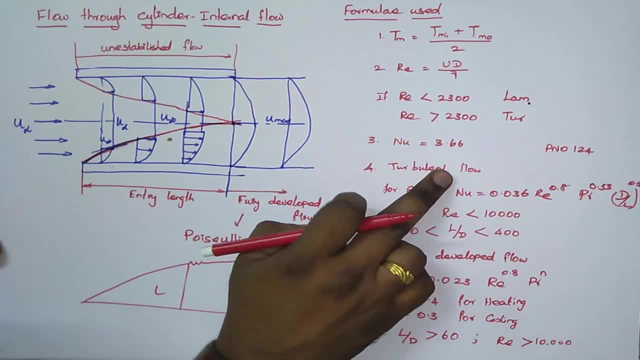 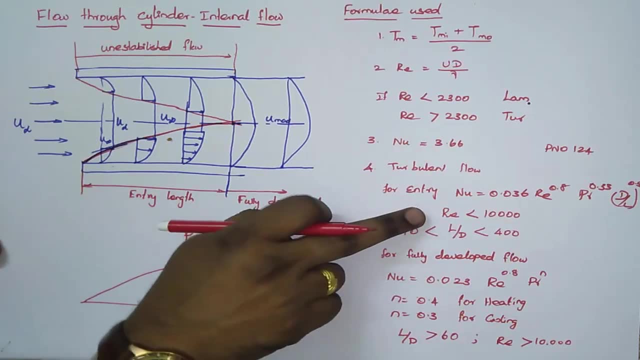 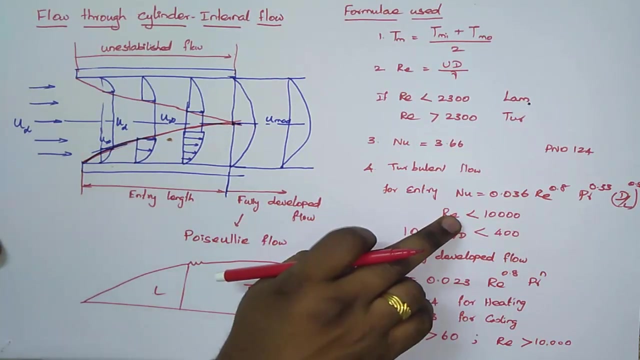 You have to assume that the flow is turbulent flow. For turbulent flow, go to page number 125 and now take the formula according to these two conditions. Now first check the Reynolds number value. If the Reynolds number is less than 10,000, then the point is in the entry region. 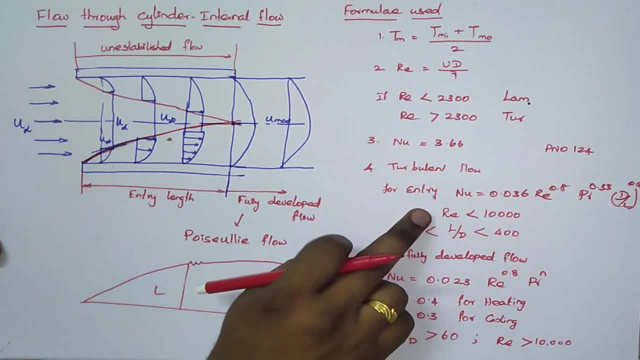 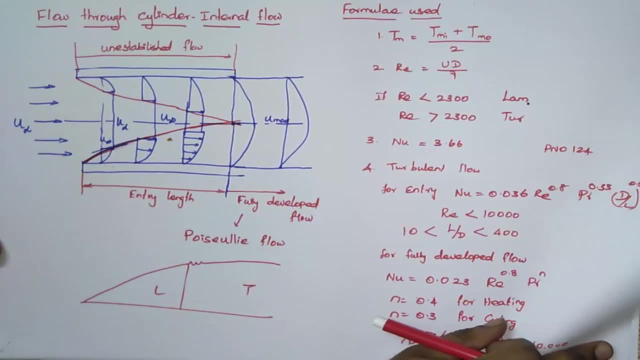 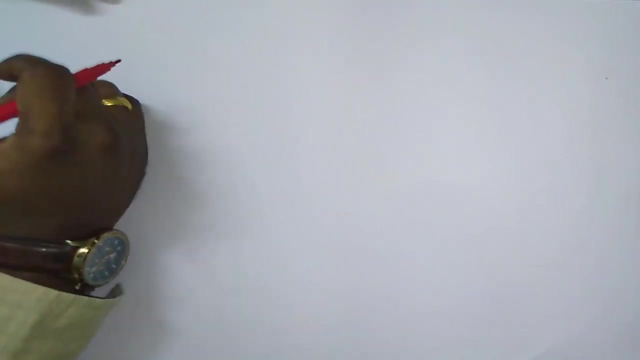 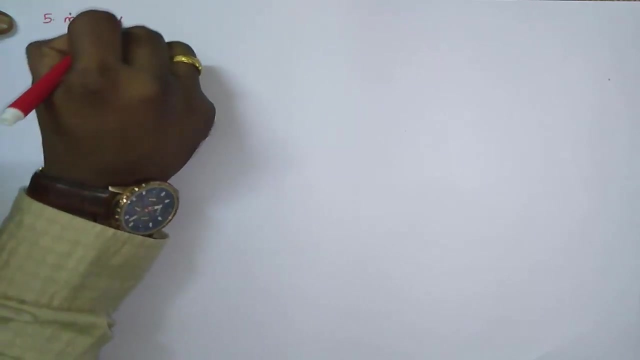 So now you just take this formula as your Nusselt number formula. If the Reynolds number is greater than 10,000, just take this formula from the data book. Okay, so the fifth formula given for solving these type of problems is fifth one. mass flow rate m dot equal to rho A? u. 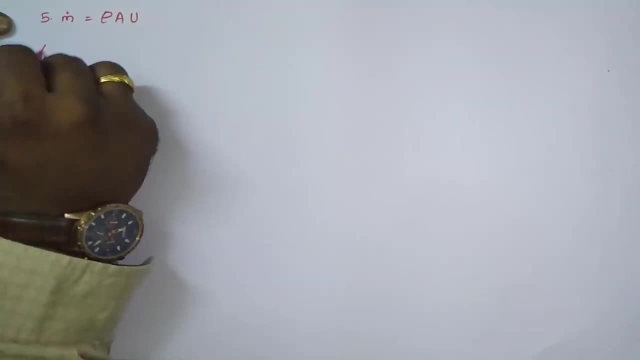 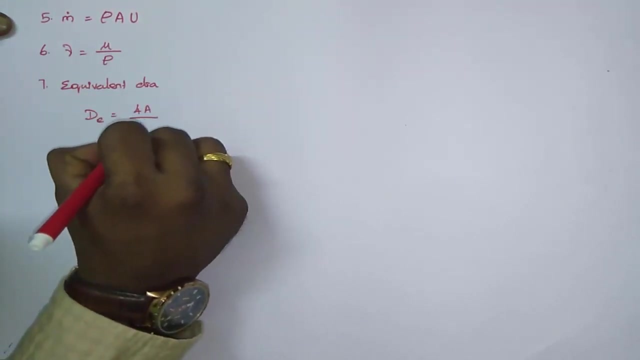 So density into area, into velocity. Sixth one is kinematic velocity: nu equal to mu by rho. Seventh formula is equivalent diameter. Okay, the equivalent diameter is nothing but d, e equal to 4 into area divided by perimeter. So now for a rectangular tube, the area is nothing but L into W. 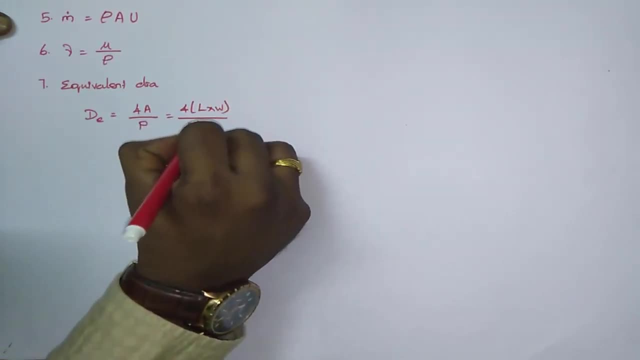 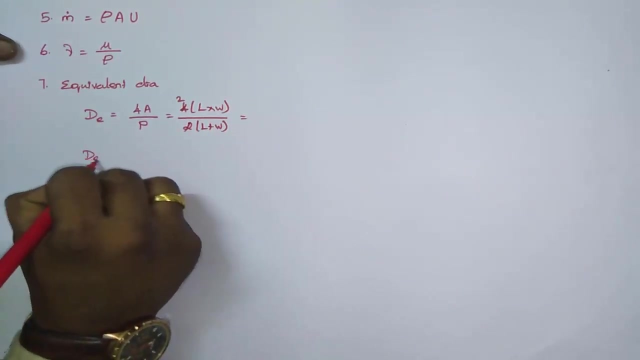 Similarly, the perimeter is nothing but 2 into L plus W, So it will get cancelled and the final value will be 2 into L into 2, L into W divided by L plus W. Similarly, the it is for rectangular tube. 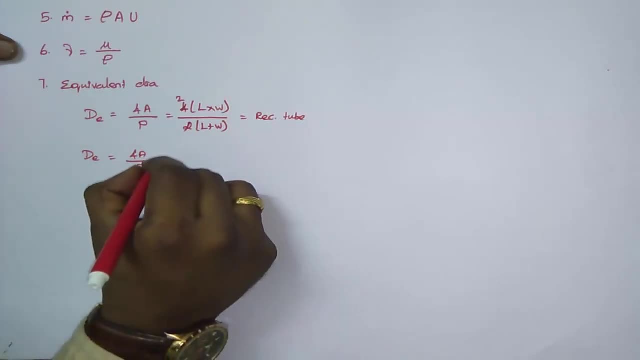 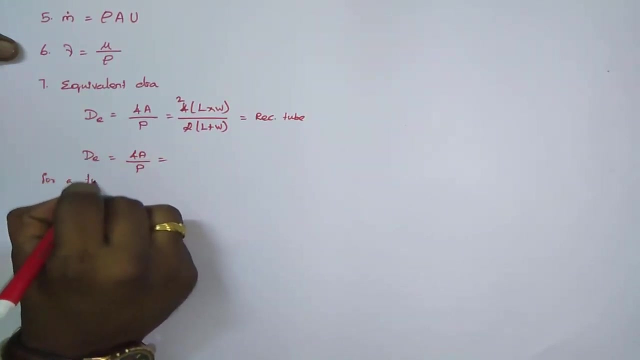 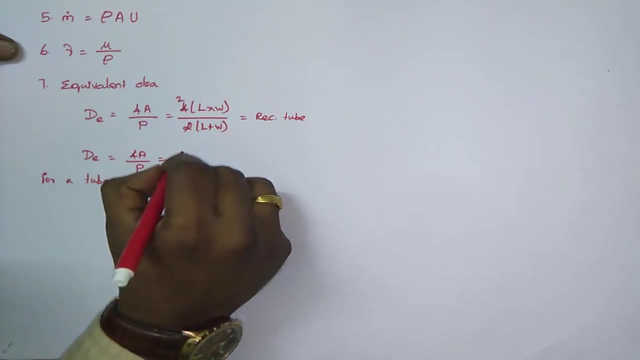 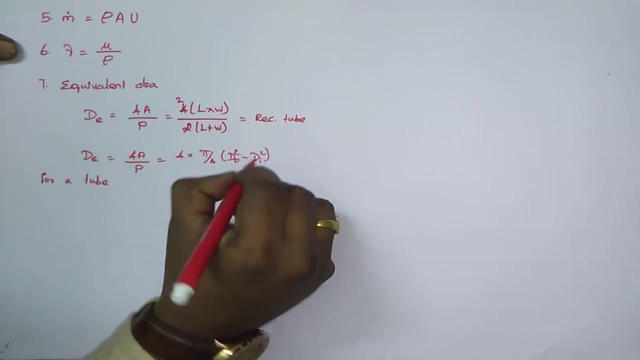 Equivalent diameter is 4 a divided by p. So for a, this is for a tube. So for a tube it will have outer diameter and inner diameter. Now the area is nothing, but is pi by 4, d naught squared, minus d i squared. 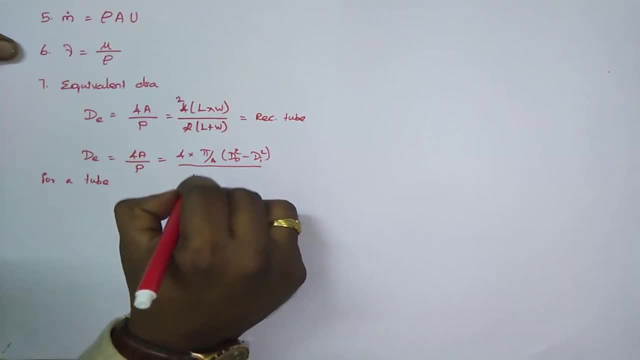 Similarly, the perimeter is nothing but pi into d naught plus d i. Okay, if you expand or if you solve these two equations, 4 will get cancelled, pi will get cancelled. Then you will get d naught minus d i as your answer. 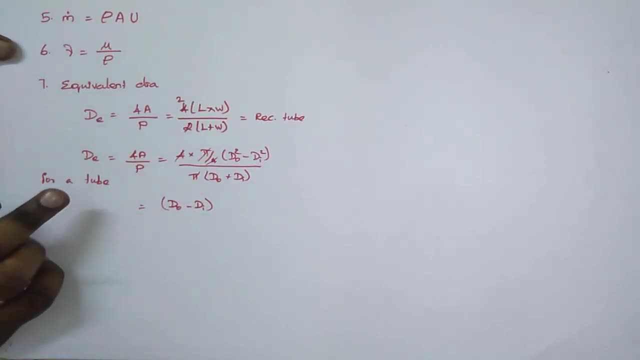 Okay, For a tube the equivalent diameter is equal to d naught minus d i. So the eighth formula is heat transfer q equal to. you know that, h a into t, w minus t mean, which is also equal to m, c, p, del t, t m naught outlet temperature minus t m i inlet temperature. 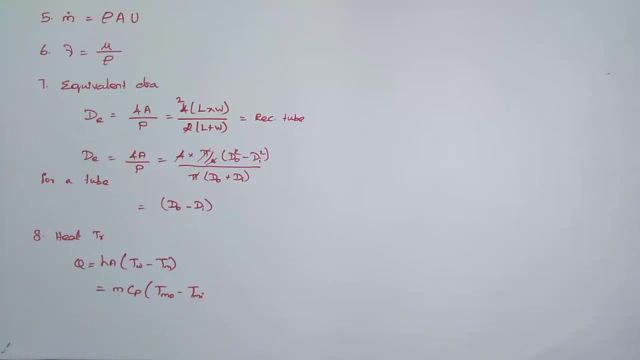 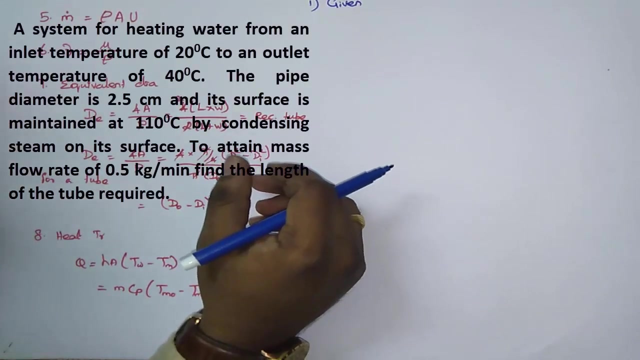 Okay, these are all the formulas You are going to use in the internal flow. Now we will solve one problem, Okay. in the first problem it is given a system for heating water from an inlet temperature of 20 degree Celsius to an outlet temperature of 40 degree Celsius. 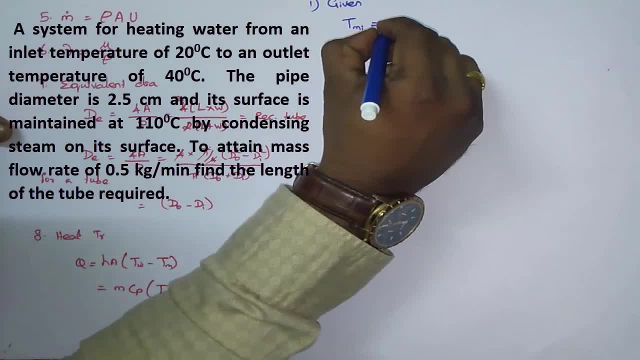 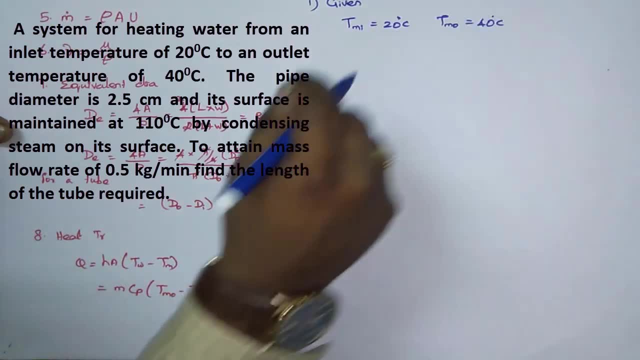 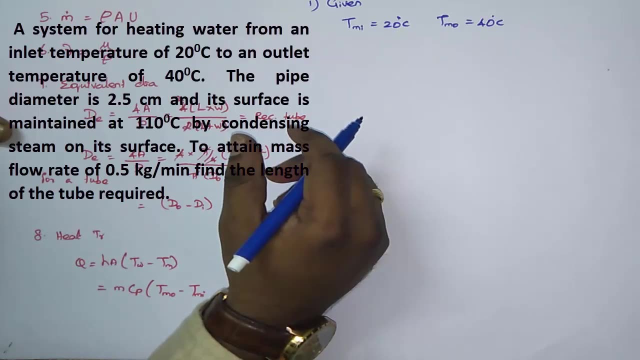 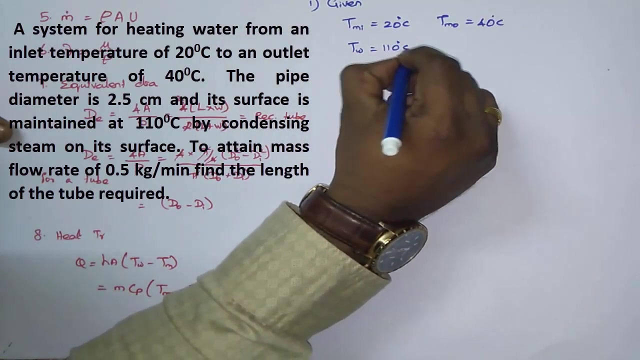 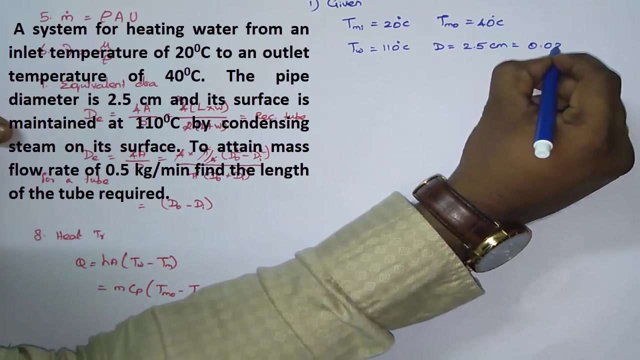 So t m inlet temperature is equal to 20 degree Celsius, t m outlet temperature equal to 40 degree Celsius. The pipe diameter is 2.5 centimeter and it is maintained at 110 degree Celsius. So pipe temperature is 110 degree Celsius and the diameter equal to 2.5 centimeter, which is equal to 0.025 meter. 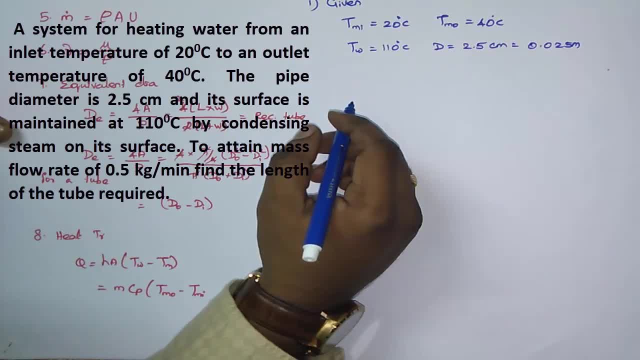 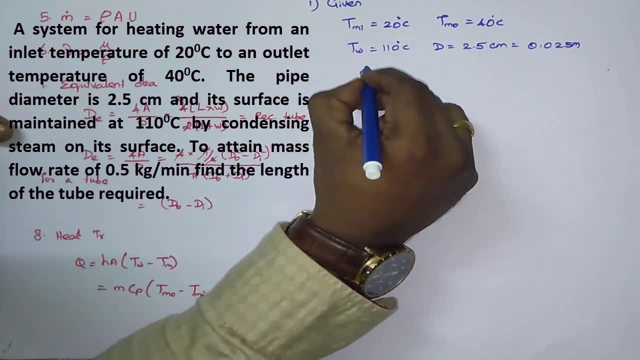 And by condensing steam on its surface to attain the mass flow rate of 0.5 kg per minute. right So m dot equal to 0.5 kilogram per minute, which is equal to 8.5 kg per minute. 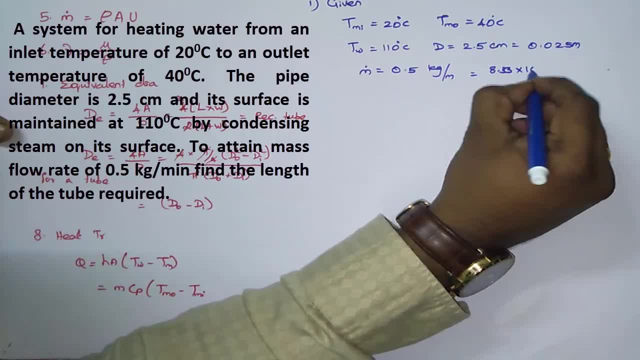 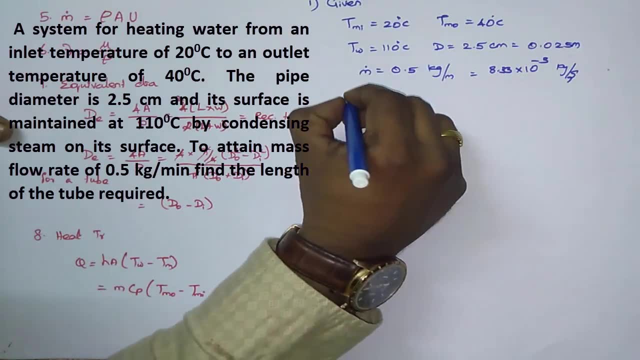 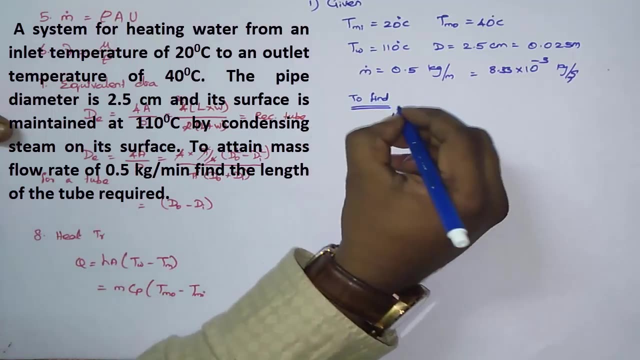 Okay, equal to 8.33 into 10, to the power minus 3 kilogram per seconds. okay, Now you are asked to find out, to find the length of the tube required. So, length of the tube you are going. 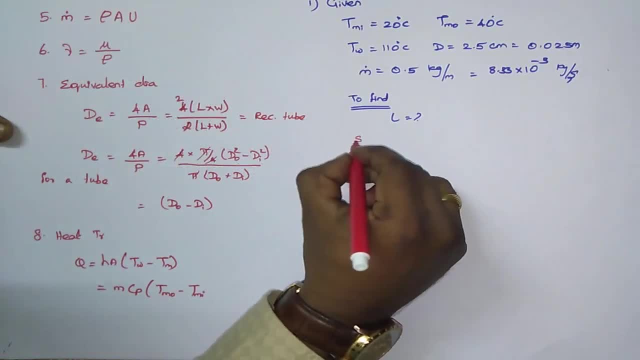 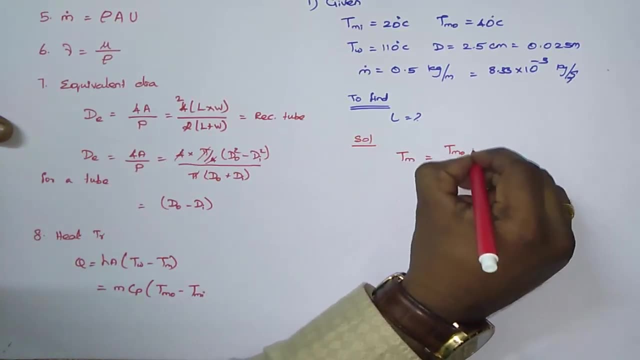 to find out Now, solution in the solution. the first step is to find out the T mean temperature, which is equal to T m naught plus T m i divided by 2, which is equal to 40 plus 20, 60 divided. 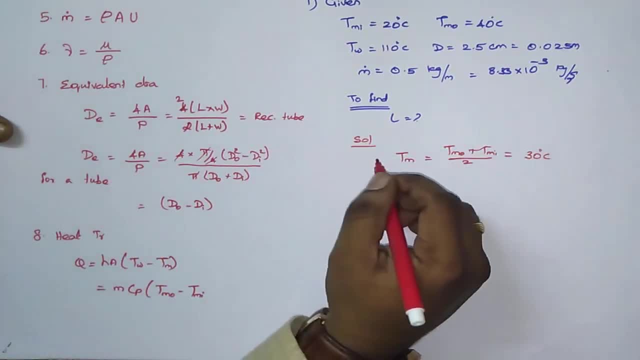 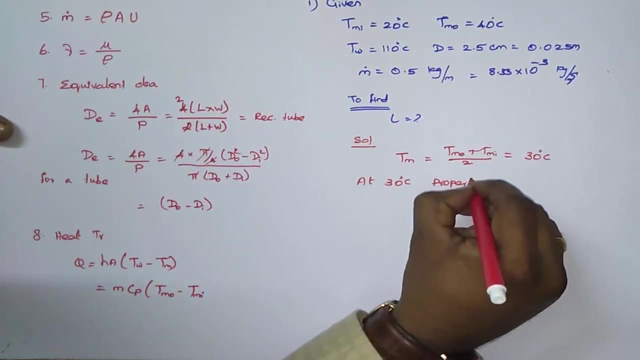 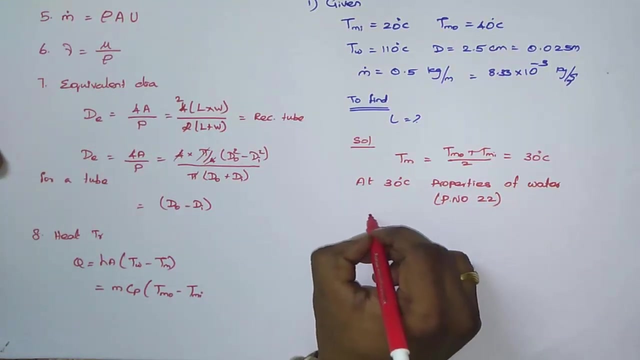 by 2, equal to 30 degree Celsius. Now, at 30 degree Celsius, properties of water from page number 22,. okay, from page number 22.. Let us take the properties of water rho, equal to 997 kilogram per meter cube Prandtl. 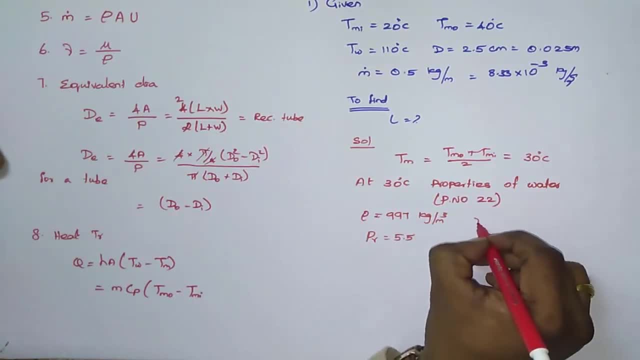 number P r equal to 5.5, kinematic viscosity nu equal to 0.857 into 10 to the power minus 6 meter square per seconds. conductivity value K equal to 0.610 watt per meter. Kelvin. Cp- heat cap, specific heat values. 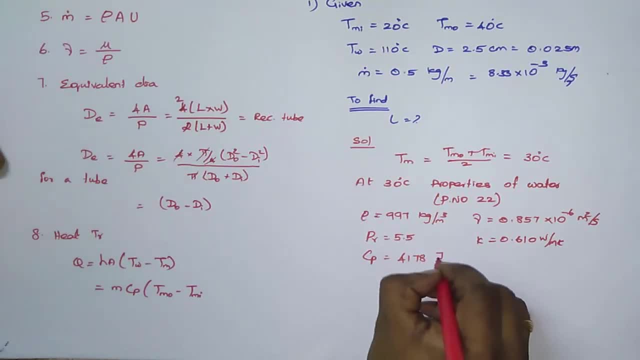 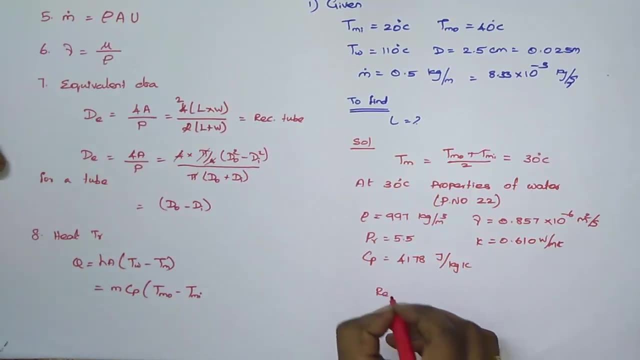 Cp- heat cap- specific heat values. Cp equal to 4178 joule per kilogram Kelvin right. This is the first step And the second step, just find out the Reynolds number value. Since it is a cylinder, you just use U, D divided. 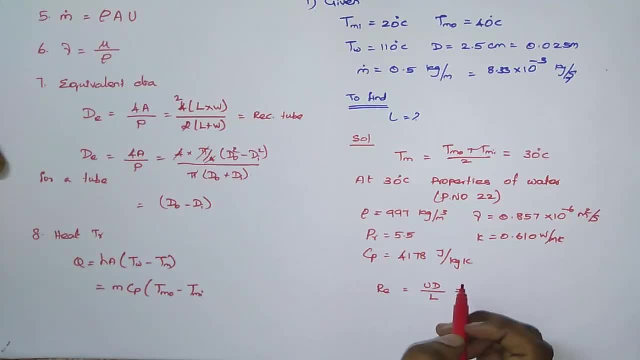 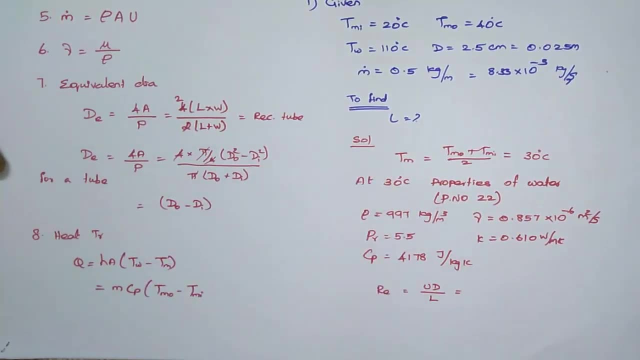 by L? U is nothing but your velocity value. The velocity value is not given in the problem. Instead of velocity value they gave the mass flow rate value. So you know that mass flow rate m dot equal to 0. So the mass flow rate m dot equal to rho A, rho A? U. From this equation you just find: 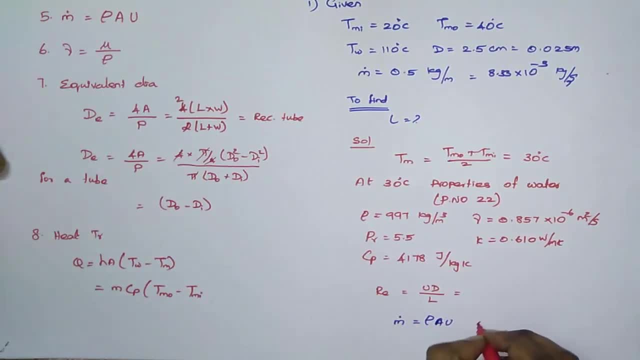 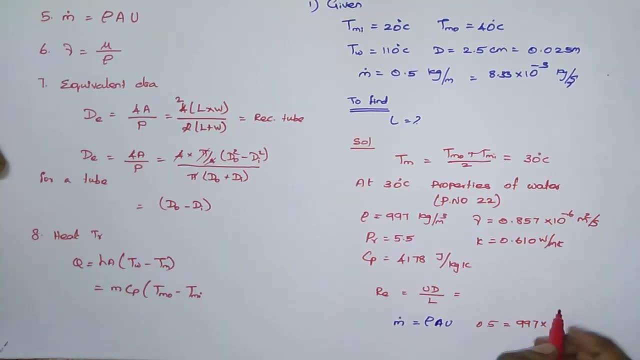 out the U value. So this mass flow rate is 0.5, you know, which is equal to 997 into the area value is pi by 4 D square. So here, the D value, you should use 2.5 centimeter. 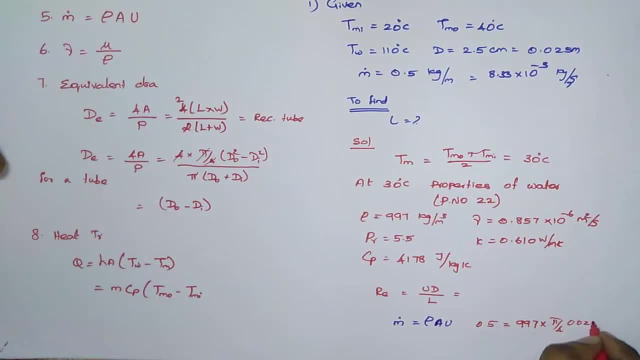 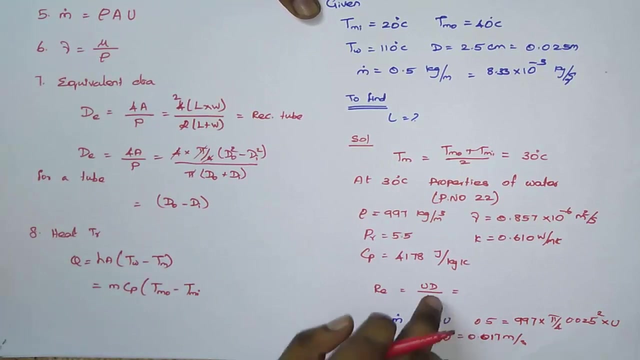 pi by 4, 0.025 square into U. From this equation find the U value, U equal to 0.017 meter per second. Just substitute this U value in this equation. you can get 0.017 into 0.025 divided by length. is sorry. 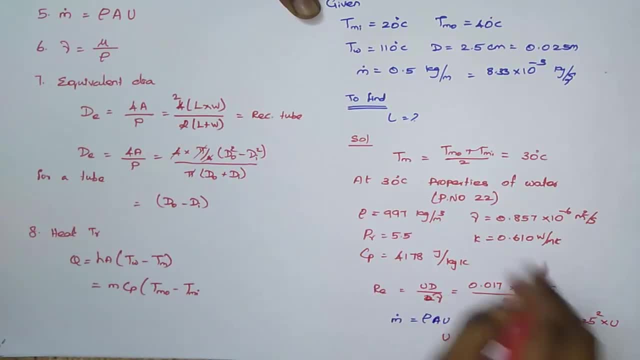 U D divided by nu. no, Here nu value is. here you can take 0.025.. meters per second Here. here you can say 0.026I. So for this you just multiply it by 0.024.. 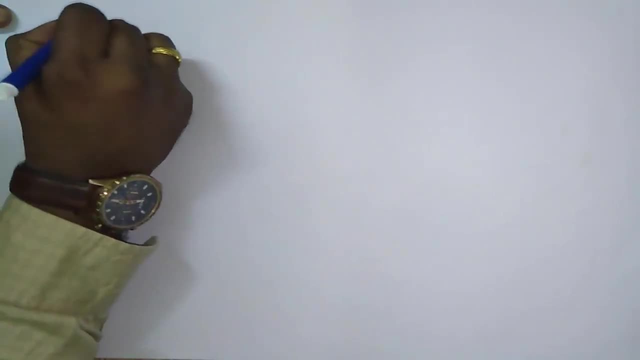 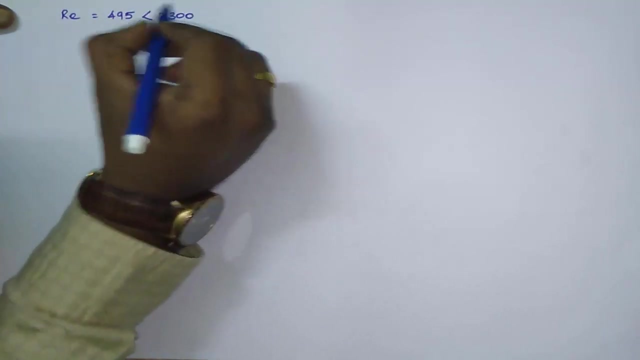 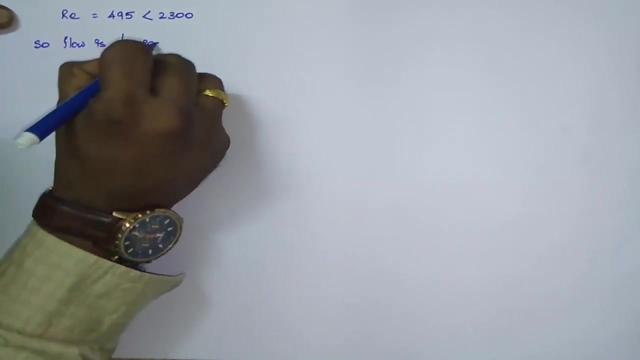 So plainly this will be the mass flow rate: 0.025 material. So you have obtained the mass flow rate at this stage. That is trairler's cost And here 0. perfektionn and here times the mass flow rate. We are taking the mass flow rate from u to that. 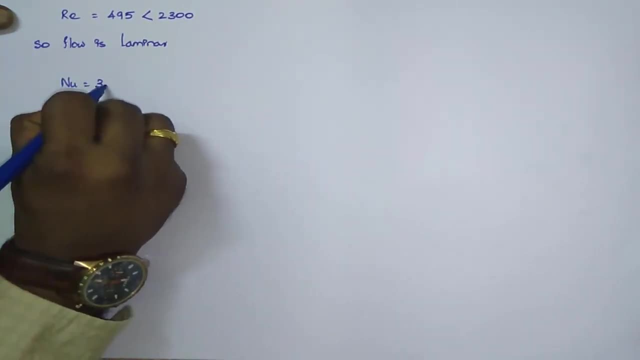 Now you will be knowing what is the mass flow rate of thisdasla notion. the smallest mass value of any material For laminar flow, Nusselt number equation is 3.66, right, So you know that nu equal to hd divided by k. okay, 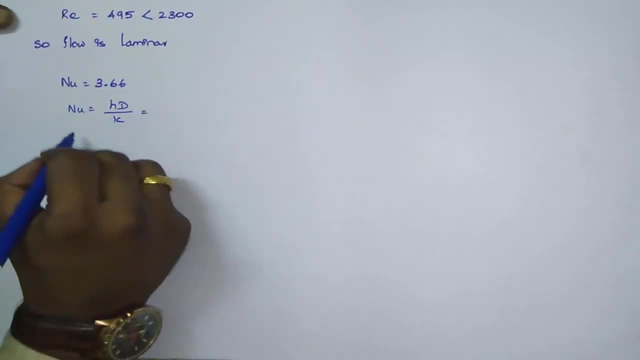 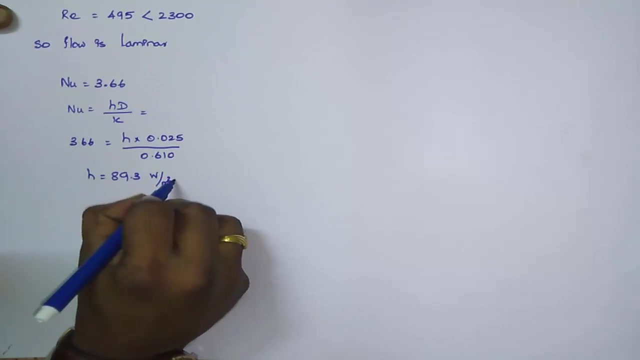 From this equation just find out. So 3.66 equal to h into diameter, is 0.025. divided by the value of k is 0.61, 0.610.. So you find out the value of h. h equal to 89.3 watt per meter square kelvin. 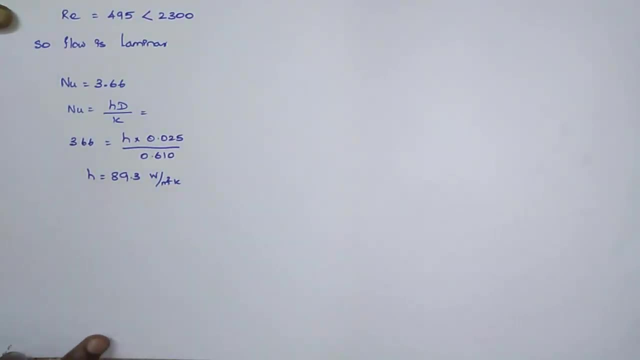 Now you have to find the value of, you have to find the length of the tube recovered. So you can find out the length of the tube from the heat transfer formula q, equal to hatw minus tm. Here the area is equal to. it is not your cross. 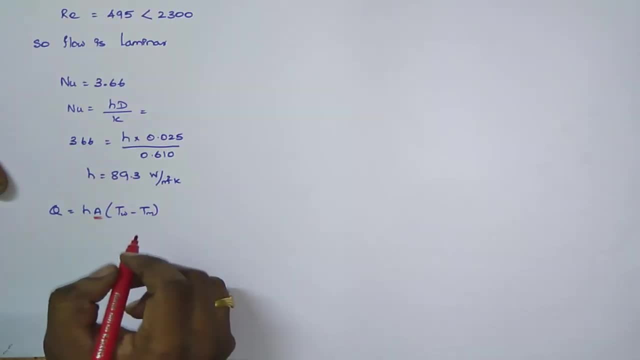 Since it is a convexion, convexion from the heat is transferred from the surface of the cylinder. So the area equal to surface area, Surface area, is nothing but perimeter into length. So pi, d into l. Here you know the value of h from here and the tw is given in the problem. 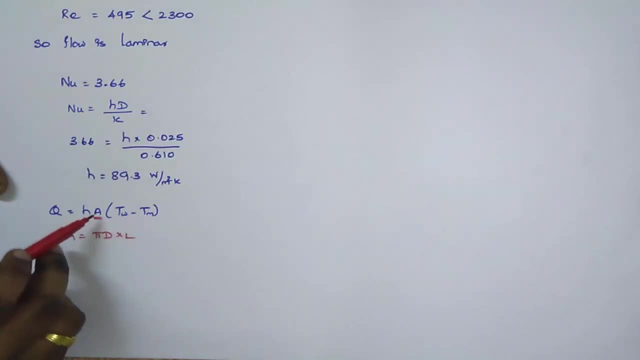 T mean temperature is 30 degree Celsius. already you find out. If you find out the area value, then from area value you can find out the length here. Another thing is you have to know the value of q. So you have the another formula for q, equal to mcp del t. Del t is nothing but tm outlet minus tm inlet. So from this equation, m equal to 0.5, into cp equal to 4178.. T outlet temperature is 40, inlet temperature is 20.. From this equation, just find out the value of q. 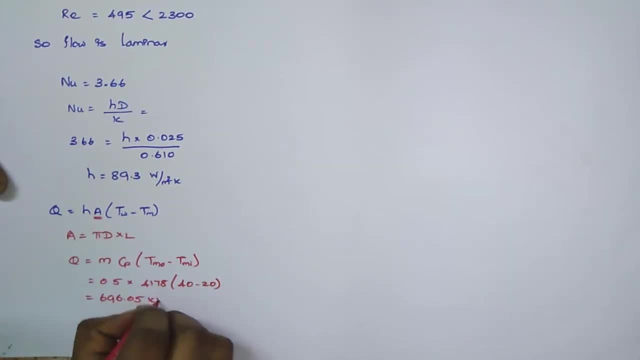 Which is 696.05 kilowatt. Just substitute this q value in this equation You can find out 696.05 equal to h into area, into tw minus t mean. Tw is 110, t mean is 30.. From this equation you can find out the value of area. 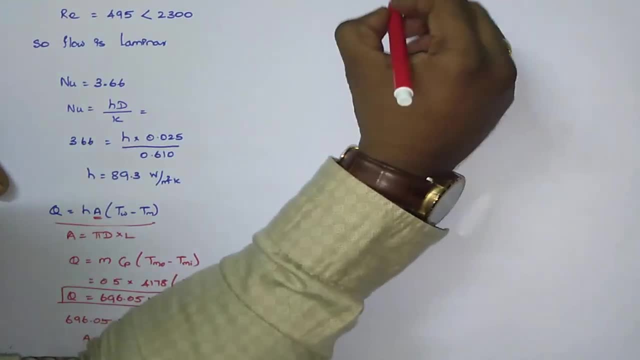 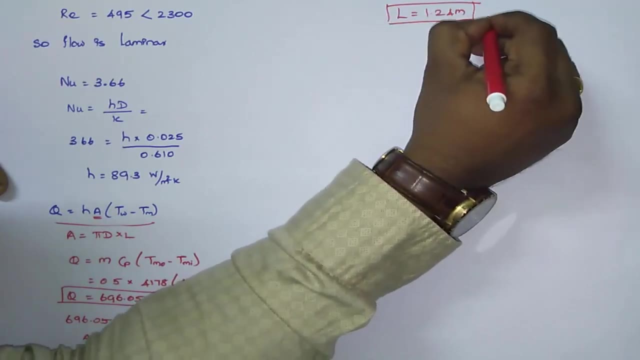 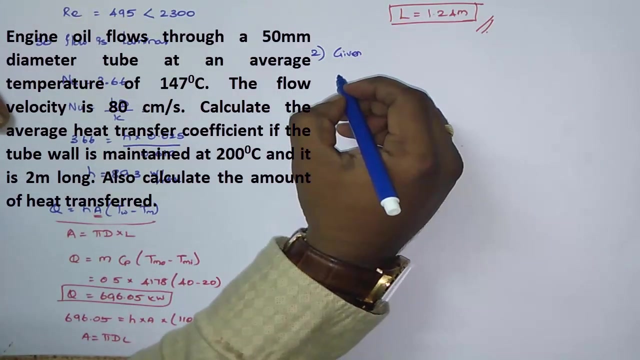 Which is equal to pi dl, That find the value of length equal to 1.24 meters. This is your final answer. okay, Now go to the second problem. Given engine oil flows through a 50 mm diameter tube, 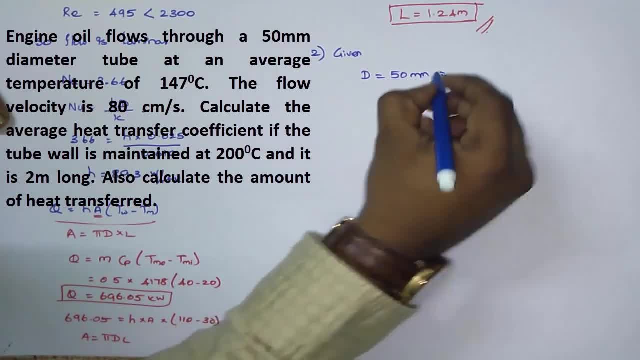 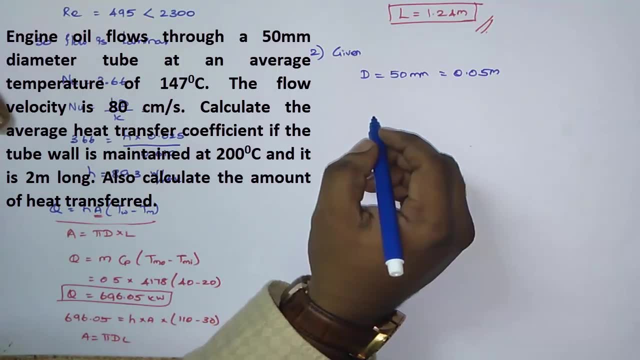 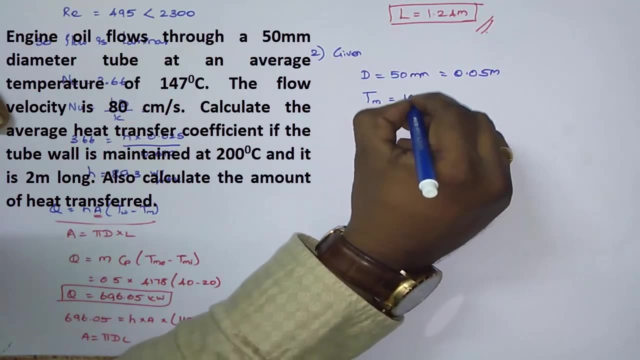 So d equal to 50 mm, which is equal to 0.05 meter, And the engine oil is at an average Temperature of 147 degree Celsius. So here, directly, average temperature is given, So t mean equal to 147 degree Celsius. 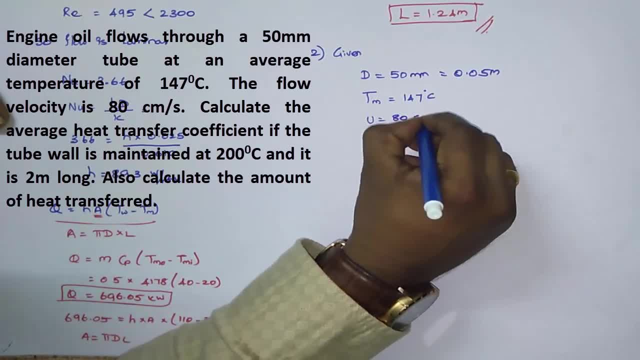 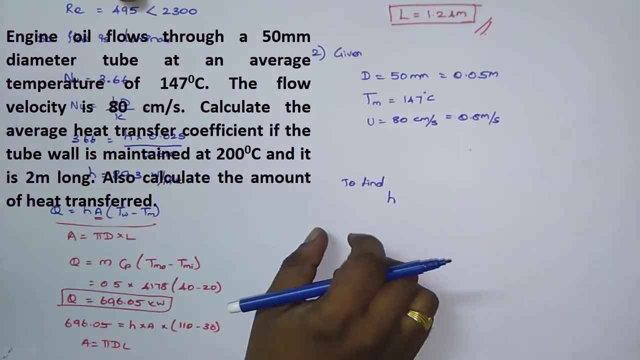 The flow velocity u equal to 80 centimeter per seconds, Which is equal to 0.8 meter per seconds. Calculate the average heat transfer coefficient to find h equal to h, And if the tube wall is maintained at 200 degree Celsius. 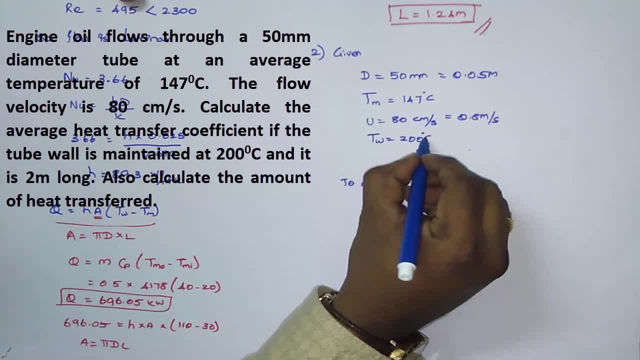 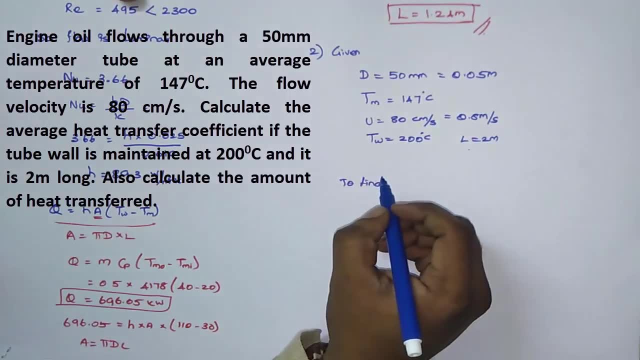 So tube wall temperature equal to 200 degree Celsius And it is 2 meter long, So length equal to 2 meters. Also calculate the amount of heat transferred. So q You have to find out the value of average heat transfer coefficient and heat transfer. 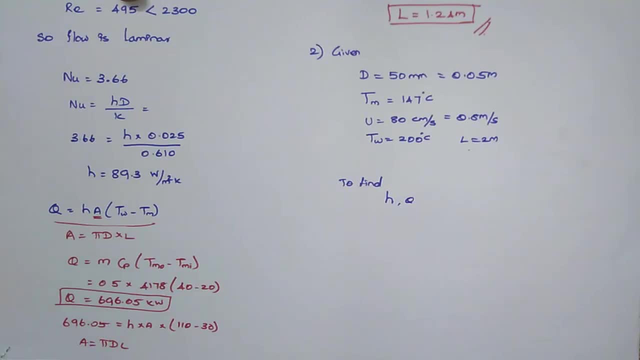 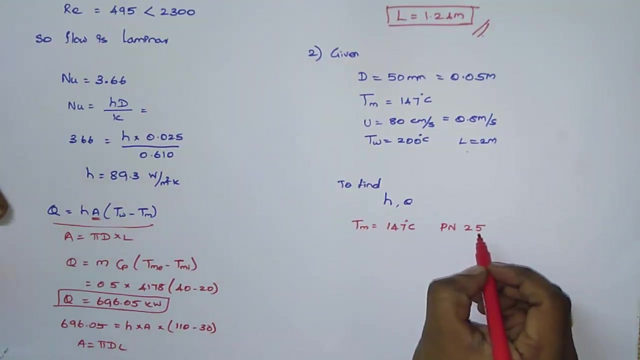 These are all the given data. Okay, In the first step you have to find out the Properties. So t mean temperature is given as 147 degree Celsius From page number 25.. In the page number 25, the properties of engine oil. 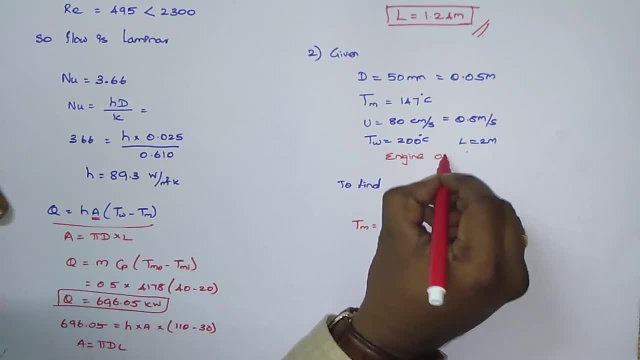 Here engine oil is used, That is, the flow liquid is engine oil. So you have to take the properties of the flowing liquid, which is engine oil. In the page number 25, you can find out the properties of engine oil at various temperatures. 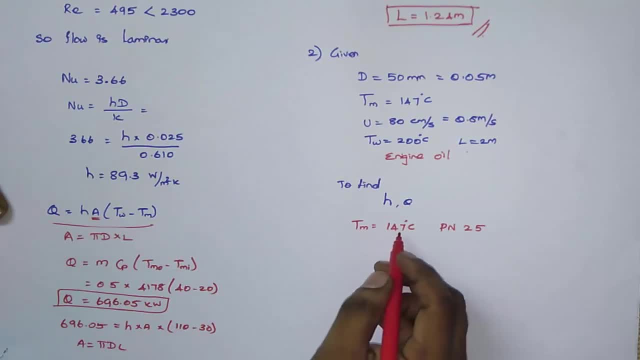 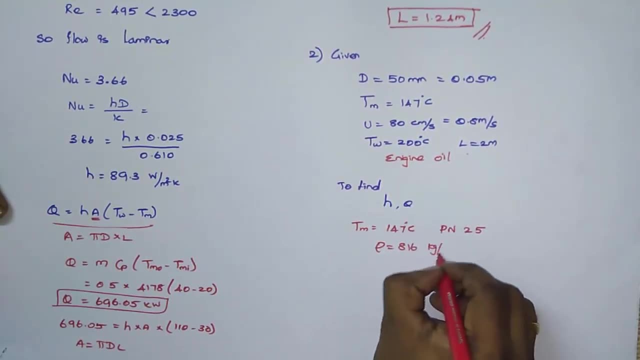 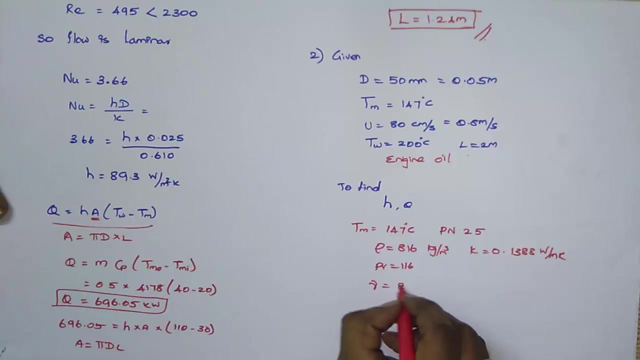 Now take the values of engine oil at 147 degree Celsius. Rho equal to 816 kilogram per meter cube, K equal to 0.1388 watt per meter Kelvin And the value of PR equal to 116.. Value of kinematic viscosity: nu equal to 8 into 10 to the power minus 6 meter square per seconds. 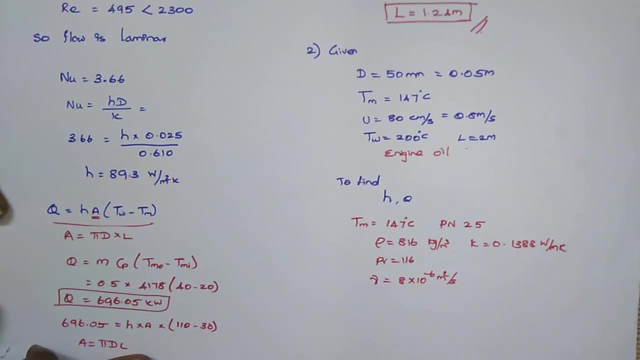 Okay, Okay, Okay, Okay, Okay. Once you find out the properties, Once you take all the property values from the data book, Then the next step you have to find out the Reynolds number. value R, e, equal to. It is an internal flow. 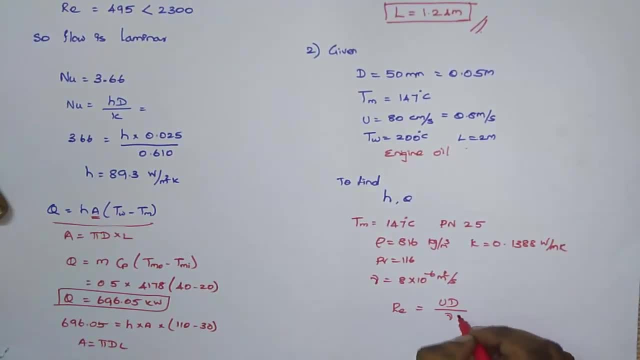 No, You have to put the formula U, D divided by nu. So U value is nothing but your 0.8.. And the diameter value is 0.05.. Kinematic viscosity value is given here 8 into 10 to the power minus 6.. 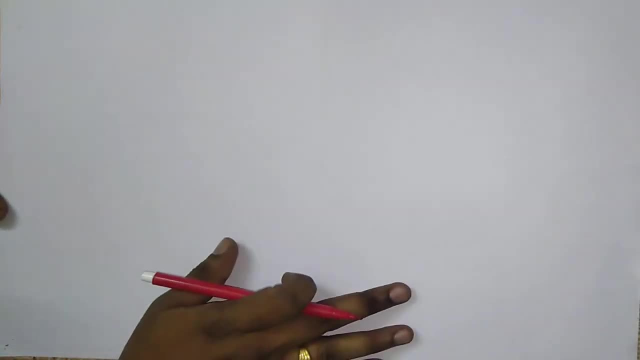 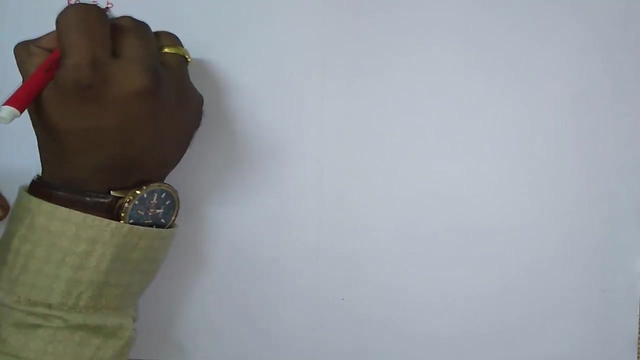 And if you Calculate the Reynolds, And if you calculate the Reynolds number value, You will get R? e equal to 5000.. Around 5000.. You will get the Reynolds number value which is greater than 2300.. So write it here. 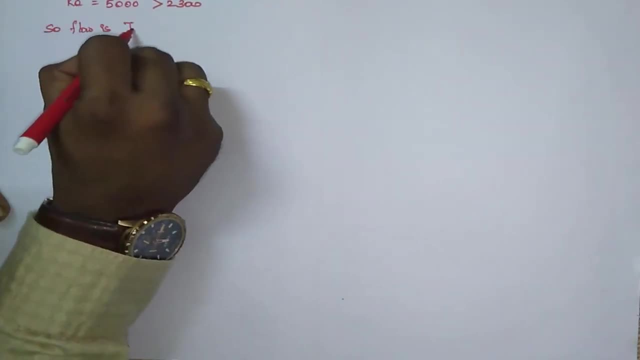 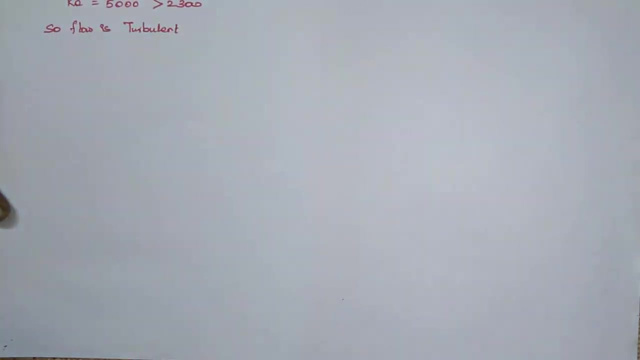 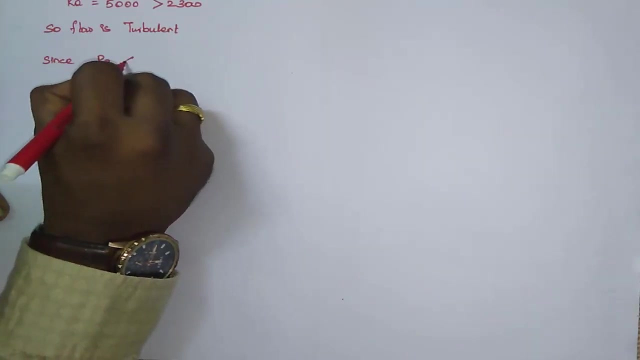 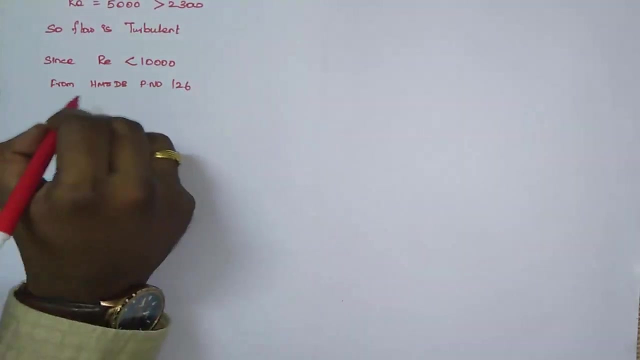 Flow is turbulent. Okay For the turbulent flow. Now you have to take the Nusselt number equation. So since R e is less than 10000, from HMT data book, page number I think 126.. No, So from page number 126, Nusselt number equal to 0.036 R e power: 0.8 PR power. 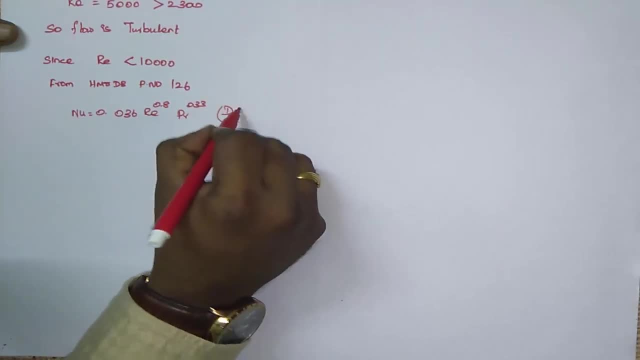 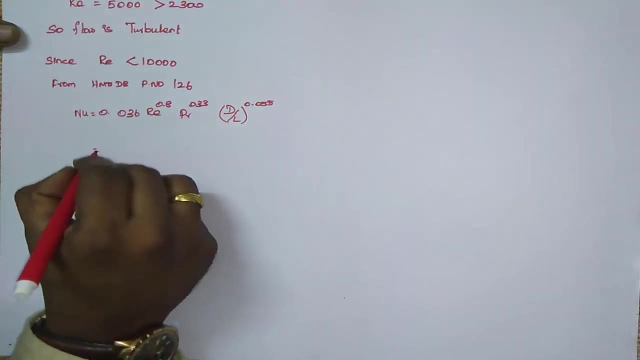 0.33 and D divided by L to the whole power 0.055.. Substitute all the values, You can find out Nusselt number is equal to 128.42.. Now this 128.42 Nusselt number equal to HD divided by K. 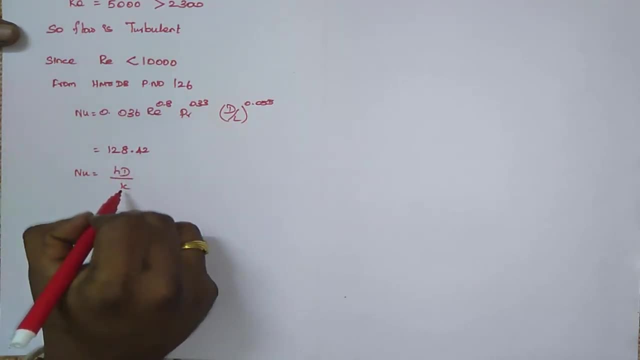 So now substitute the value of D and conductivity value, You can find out H value, That is, 343.65 watt per meter Kelvin. You know that the second subdivision. you have to find out Q value. Q equal to HA. TW divided by T mean.